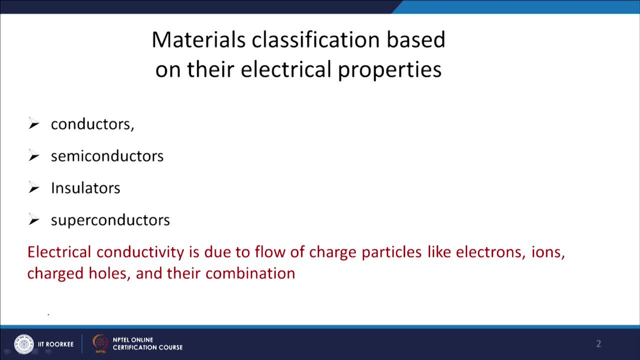 applications, and this is semiconductors. okay, so understanding semiconductor is very important. that is what we will concentrate more in this lecture. Then there are insulators. okay, of course, these are also important, because if you have a semiconductor, you have to have a insulation around that. similarly, the insulators can. 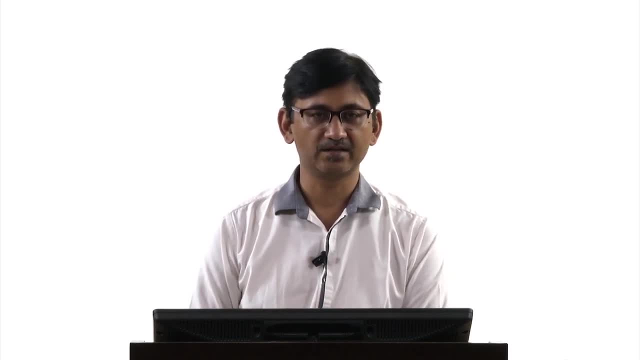 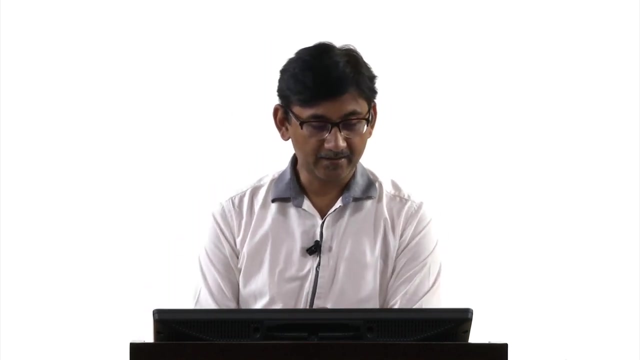 be ceramic materials, for example, usually insulator because of the covalent bonding- okay. or ionic bonding between the 2 atoms- okay. there are no free electrodes for conduction, but sometime these ceramic material can show a very important property which is called superconductors- okay. 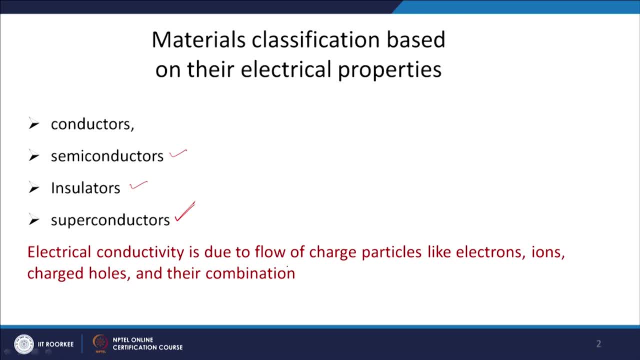 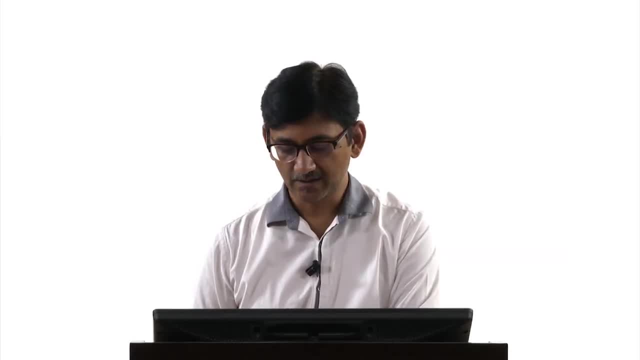 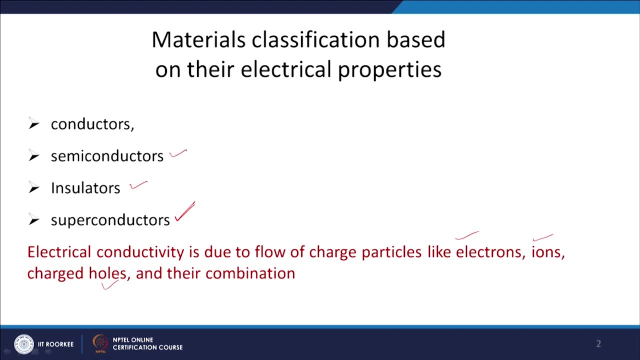 The electrical conductivity is due to flow of charged particles. okay, so any conductivity will be related to movement of charged particles. these charged particles can be electrons, or it can be ions also, or it can be charged holes. okay, so when electron leaves a valence band, 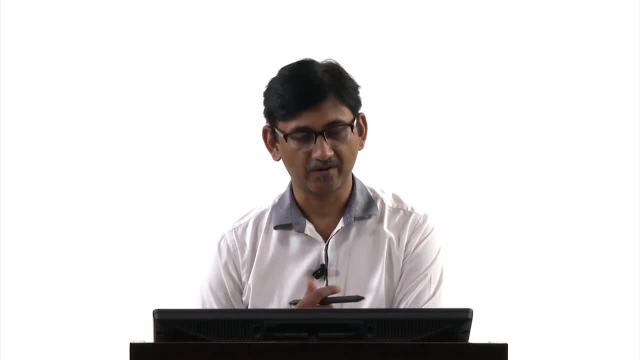 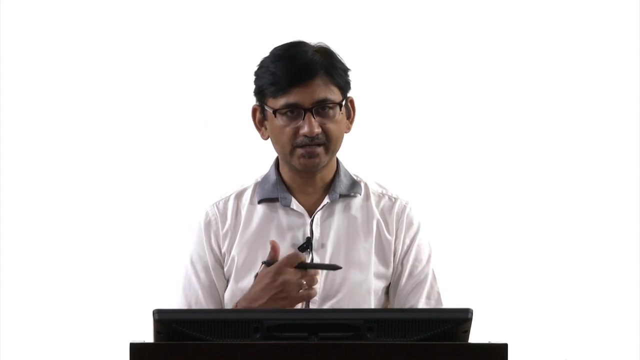 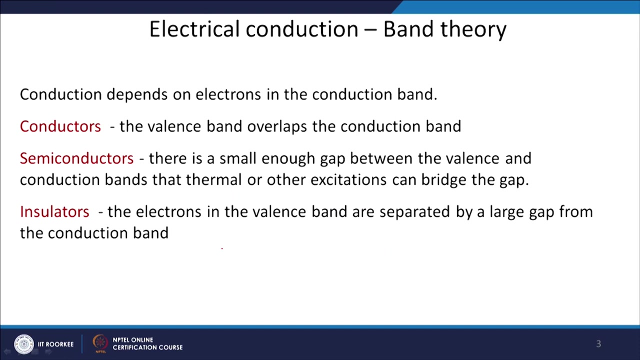 it leaves behind one hole, okay, which can be considered as positively charged hole. okay, So the conduction will depend upon the movement of these charged particles. the electrical conduction can be explained using band theory. that where the electrons are residing- okay, so in conduction depends on electrons in the 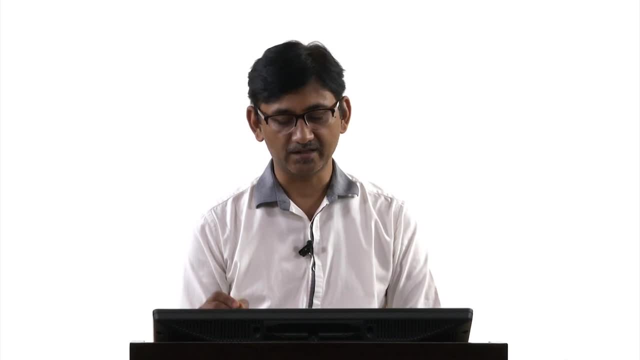 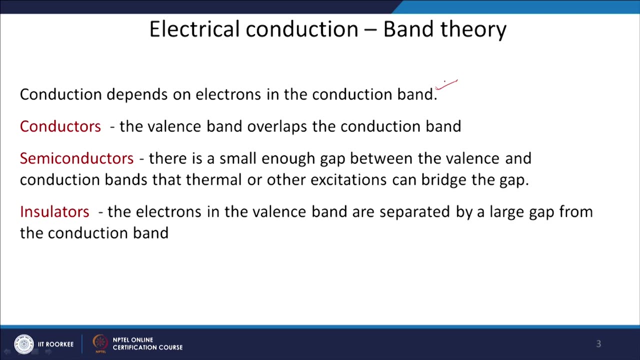 conduction band. if the electrons are in the conduction band, then you will have a conductivity, otherwise you would not have okay. So if the conduction is due to flow of electrons, so the conductors are the ones which have valence. 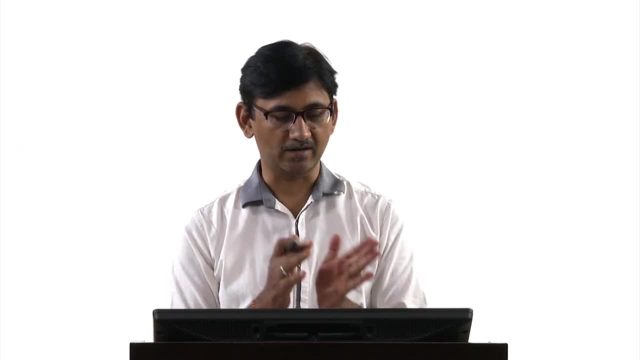 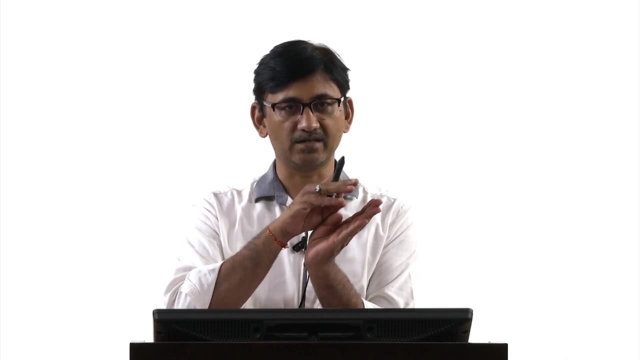 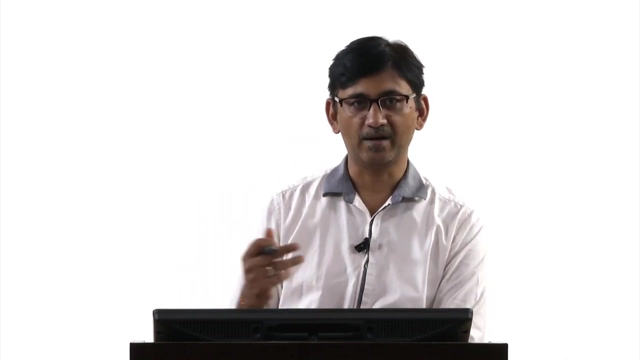 band overlapping the conduction band. so in case of conductors, what happens? the electron, the conduction band and the valence bands are overlapping each other, so the valence, the electron in the valence band can easily go to the conduction band. and when you apply, 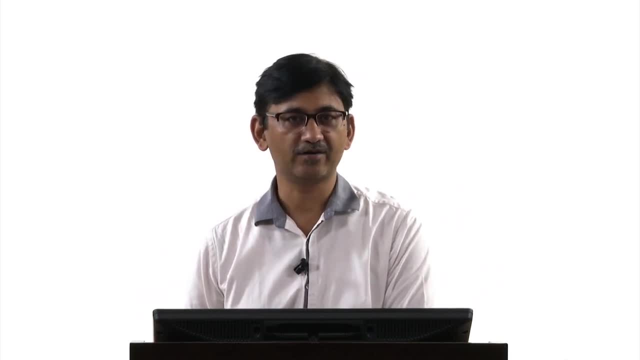 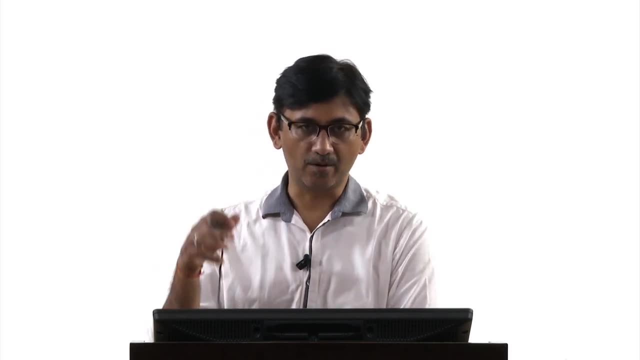 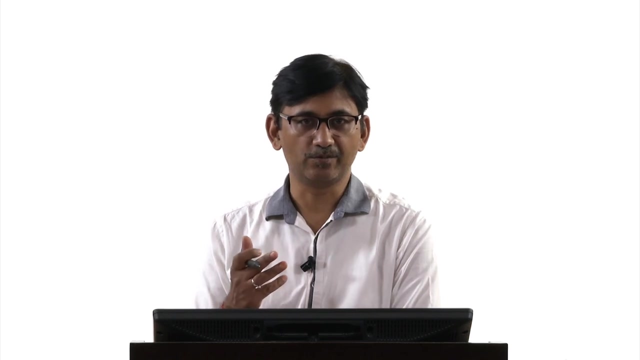 any electric field, the flow of electron will start, okay. so you have lot of free electrons there, okay, which are not bounded by the atom. okay, or they are not in the valence shell, so they are free to move around. okay, because they are in the conduction band and 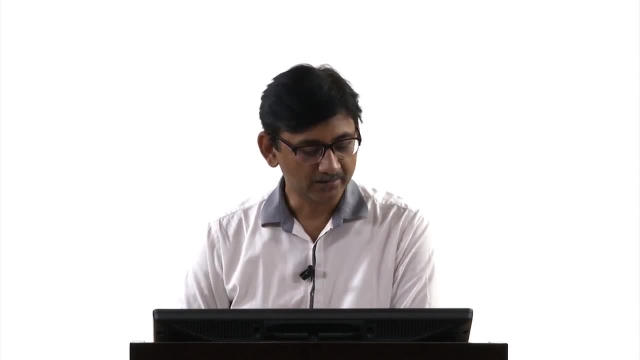 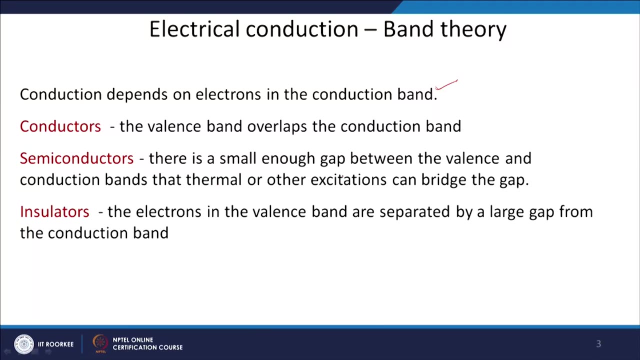 as soon as you apply any electric field, they will move. There is a small gap between the valence and the conduction band. okay, but due to thermal excitation these electron can go from valence band to the conduction band, so you can increase. 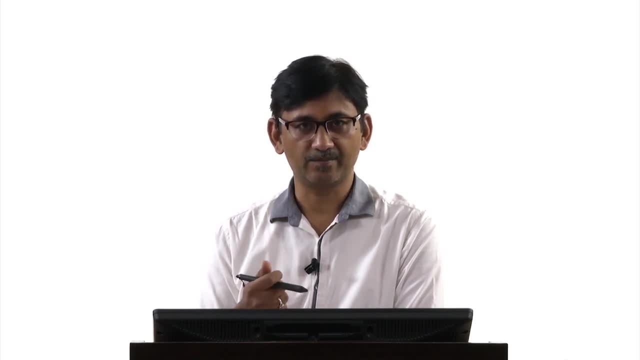 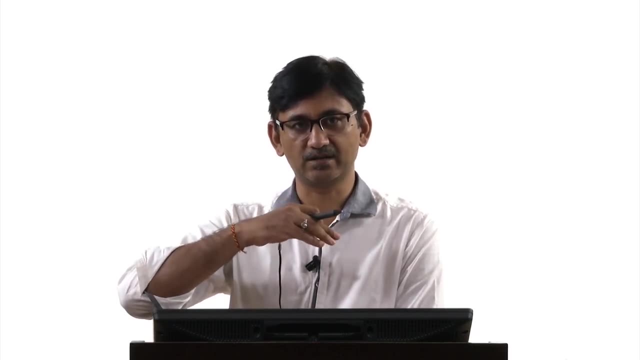 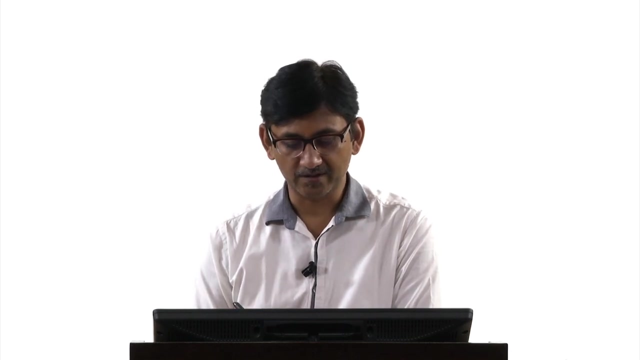 the conductivity of the semiconductor by taking it to higher temperatures, okay, where the thermal energy or the thermal excitation will push the electron from valence band to the conduction band, okay. So this is one of the important difference between the conductor and semiconductors. 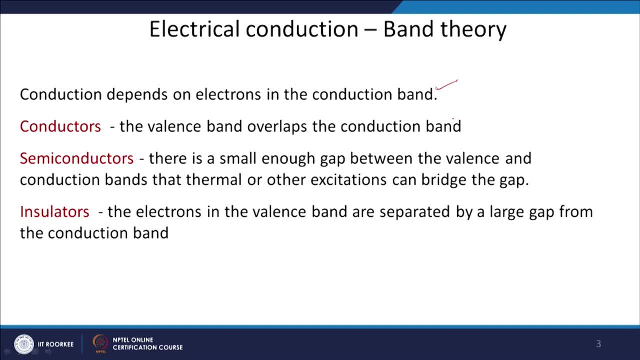 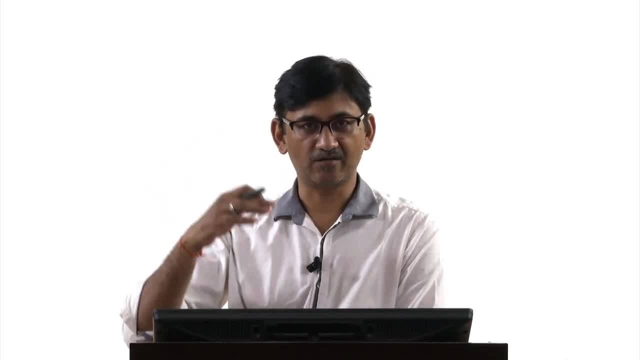 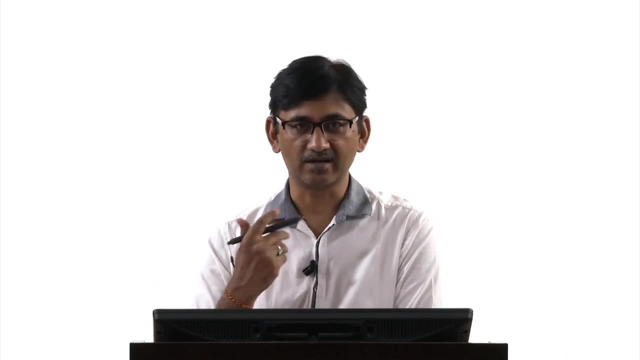 that the conductor, or the conductors, have lower conductivity at higher temperature. so as you increase the temperature the conductivity of a conductor will come down, whereas in case of semiconductors, when you take it to higher temperature the conductivity increases. okay, because now more electron can go to the conduction band. 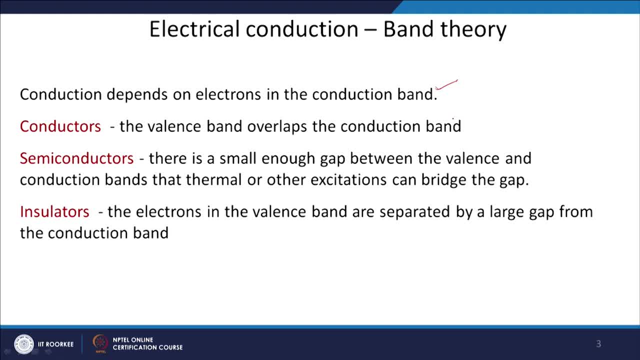 In case of insulators, the electron can go to the conduction band. in case of insulators, The electrons in the valence bands are separated by a large gap from the conduction band. okay, So between valence band and the conduction band there is a very large gap, okay, and they? 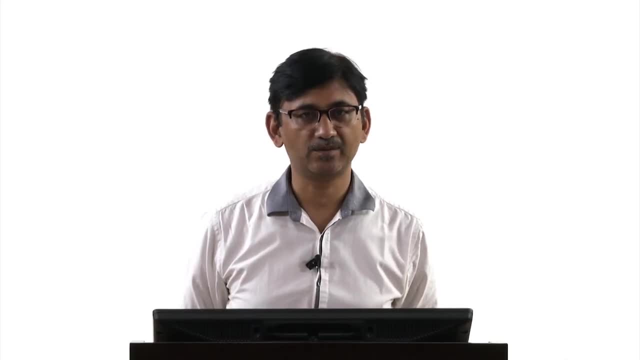 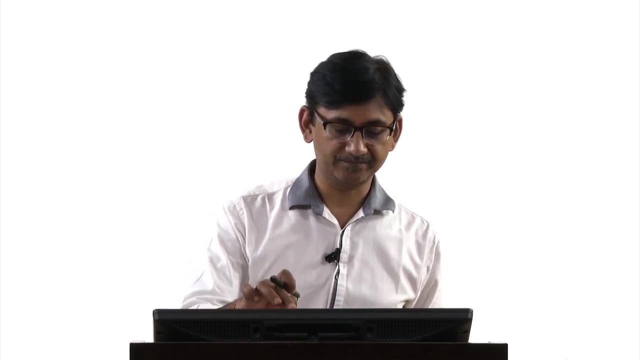 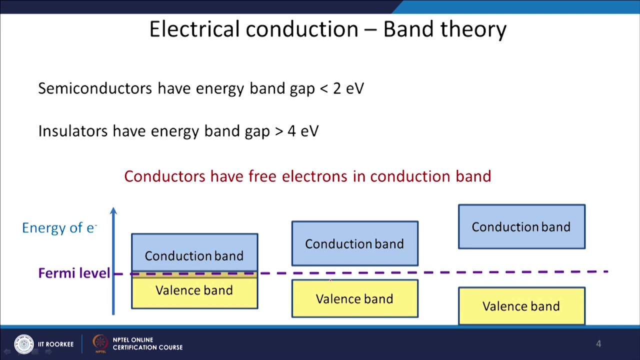 cannot jump from valence band to conduction band. so that is why insulators do not conduct any electric charge. So this is how, if you see in terms of a graph, okay, that how these different bands are there, so conduction band and valence band are there. 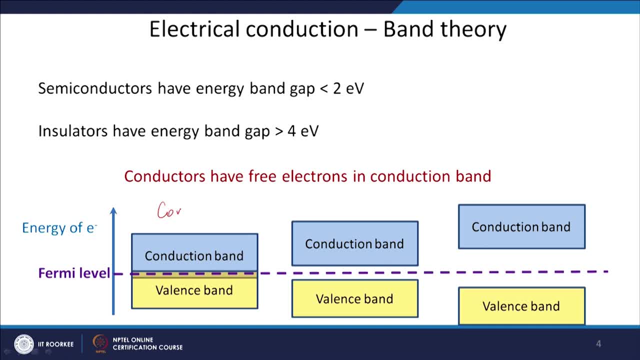 So in this case, this is the case for conductor. okay for conductor. the two are overlapping each other. so the electrons in the valence band can easily go to the conduction band, okay, and they can carry the charge okay when an electric field is applied, whereas in semiconductors, 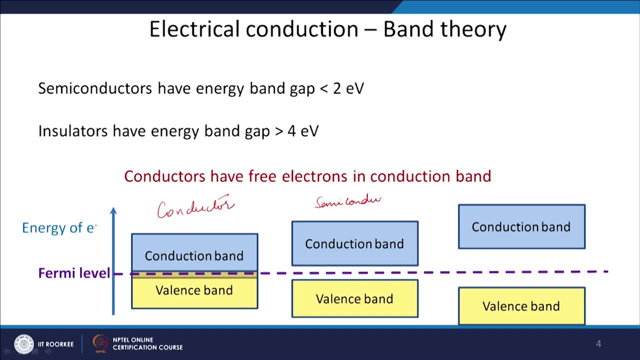 so this is for semiconductors. Okay, So there is a small gap between the valence band and the conduction band, but the gap is quite small so that if you have any thermal excitation, the electron can jump to the conduction. 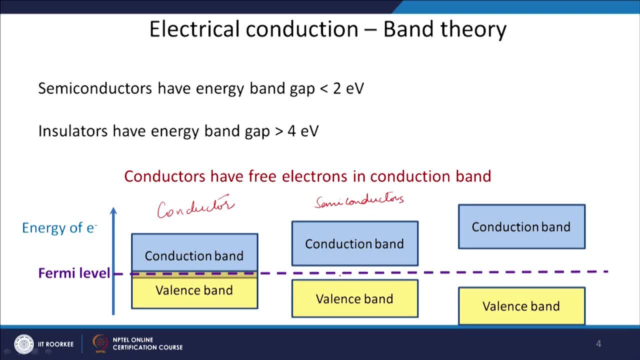 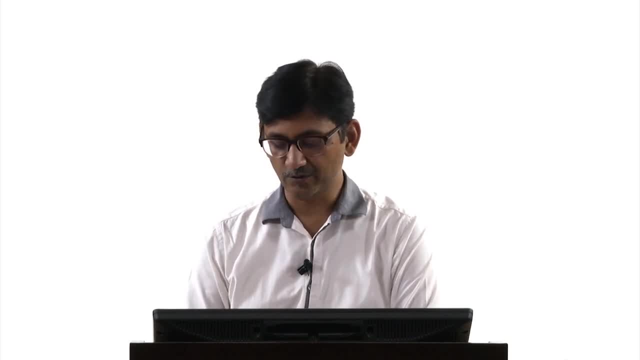 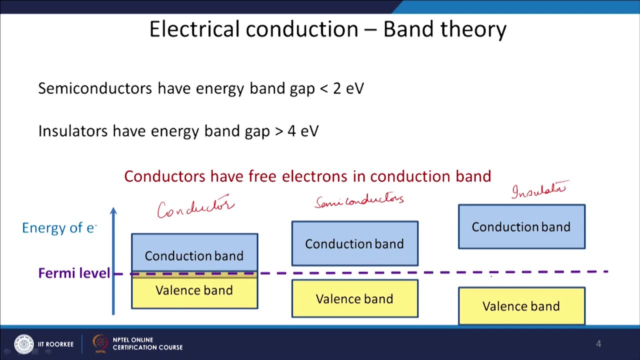 band. So at 0 Kelvin of course no conductivity will be there, okay. but at any higher temperature this conductivity will start increasing. in case of insulator, so this is for insulator. you will have a large gap between the two and it will not be able to for electron to. 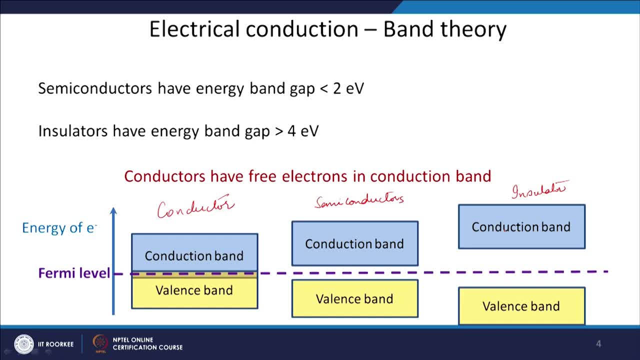 jump to the conduction band. okay. So if you want to see the energy gap in terms of some values, semiconductors have energy band gap of less than 2 electron volts, whereas insulator have energy gap of more than 4 electron. 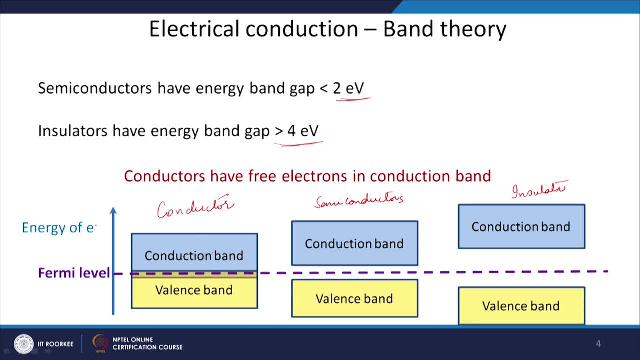 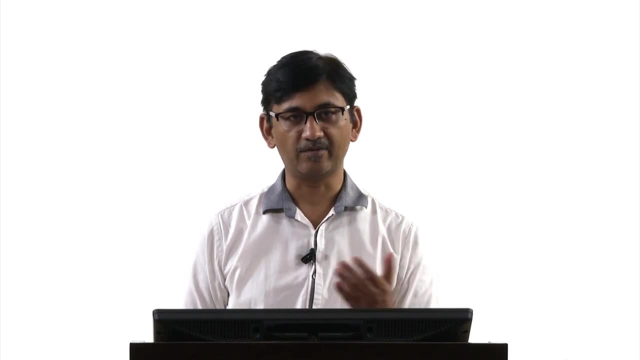 volts. okay, in case of conductor, they are overlapping each other, so there cannot be any gap. Okay, So on Y axis, the energy of electron is there. so this is what is the band theory to explain the conduction in different type of material, that why you have conduction in some material. 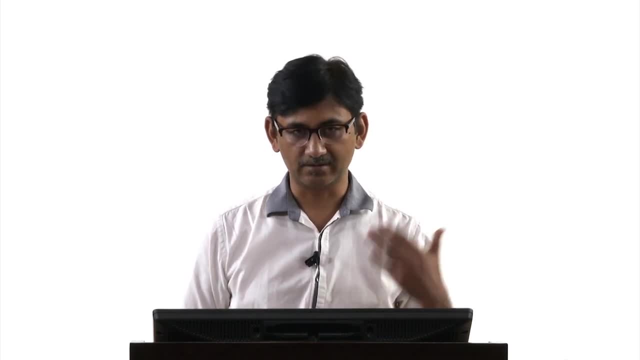 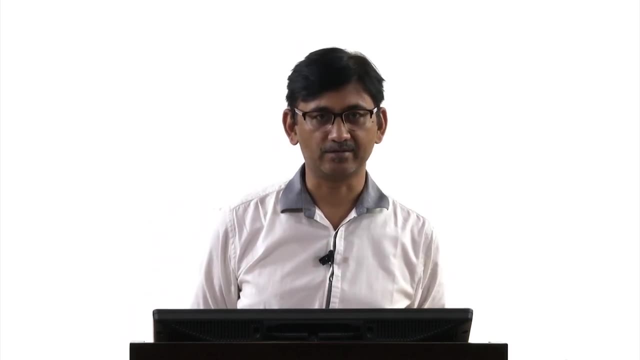 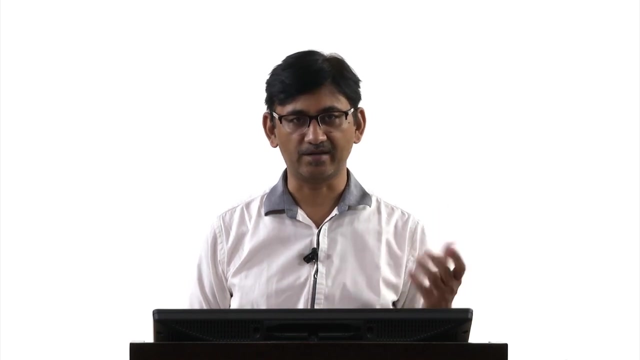 and not in some other materials. okay, Of course, the theory is much more. you have to understand more of that: how the electrons are positioned, Okay, How the electrons are positioned in an atoms, in shells, in subshells, and there is spin. 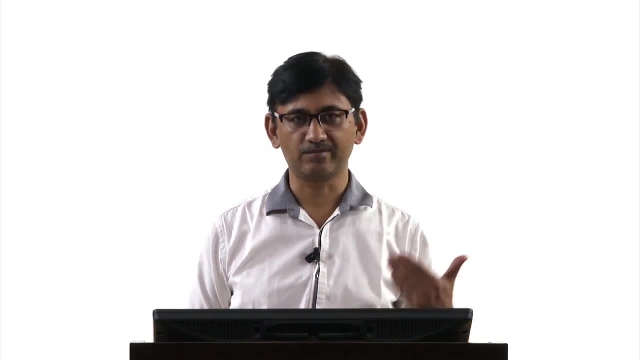 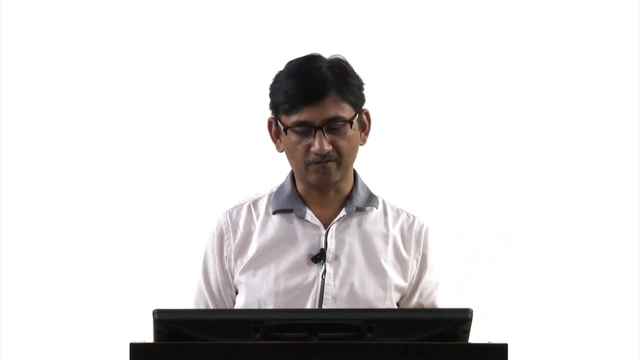 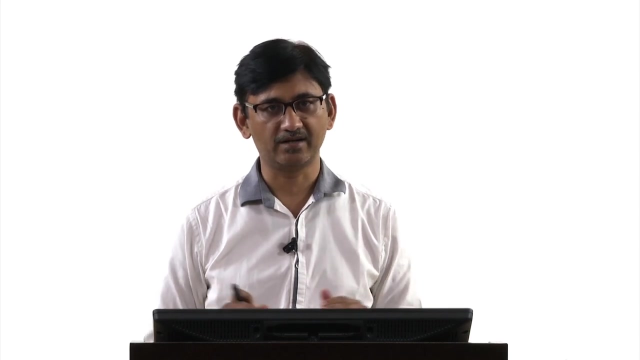 associated with each electron and so on. so those are. you have to go into much more details if you are interested only in the electrical properties of the material. okay, For our purpose right now, this much information is sufficient to understand that we can have different type of materials and how the conductivity of different materials can change as a function. 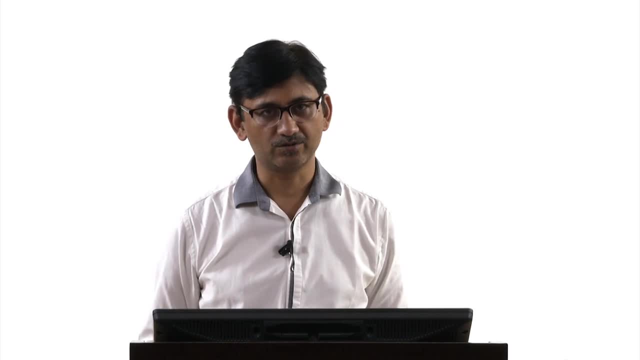 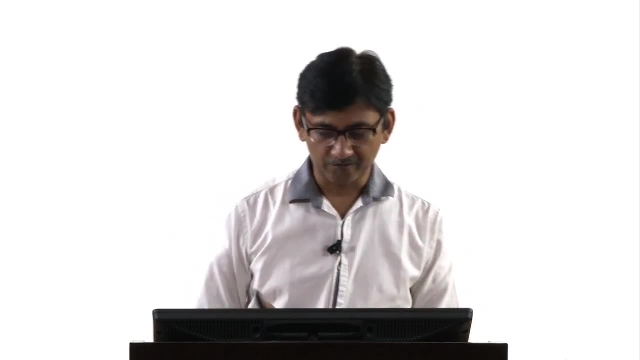 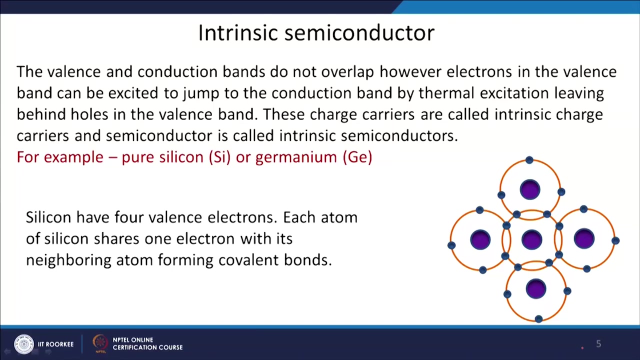 of temperature, for example. there are other ways also to change the conductivity of the material and that is what we will see in the next slides. So if you come to semiconductor, semiconductor, we will look slightly in detail because these are more one of the most important materials. in fact, all the electronic industry is based. 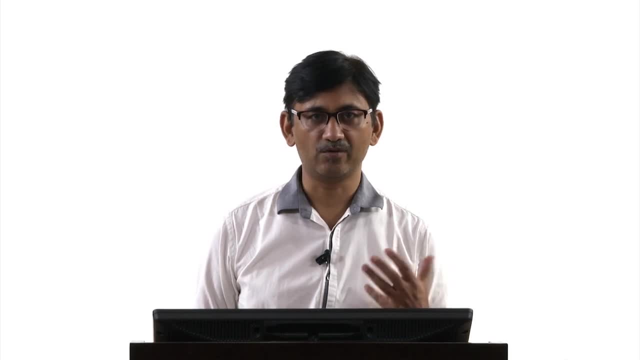 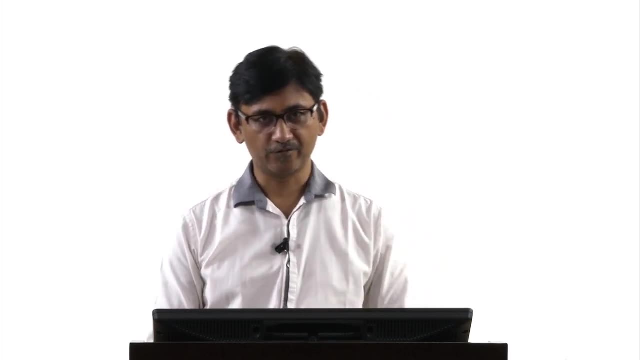 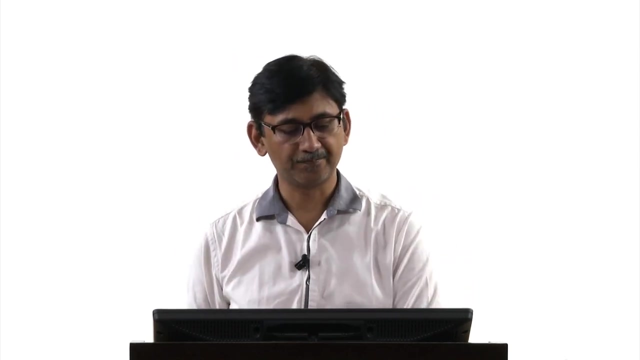 on only on the semiconductors. okay, that how you can manipulate the properties of the semiconductor. So if you look at the semiconductor, there are can be of two types. one is what we call as intrinsic semiconductors. okay, 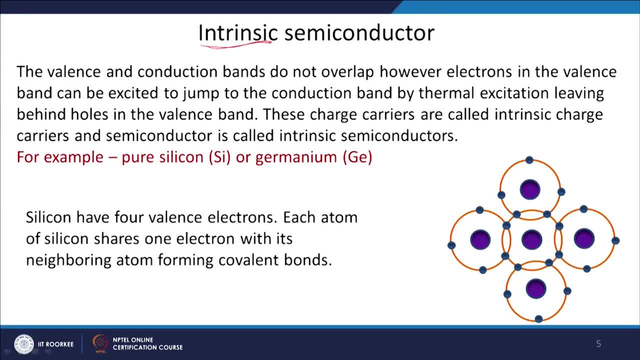 So in case of semiconductor the valence and conduction bands do not overlap, okay. however, electrons in the valence band can be excited to jump to the conduction band by thermal excitation, leaving behind holes in the valence band. okay, so when the electron goes from, 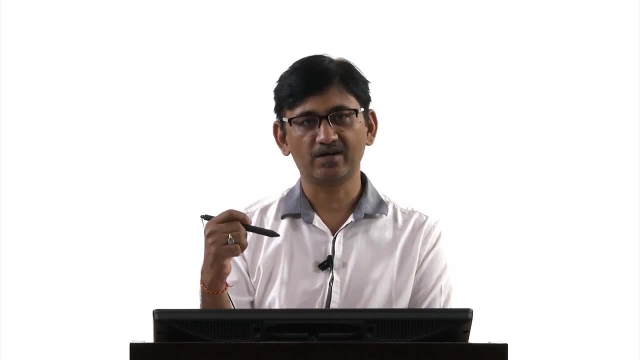 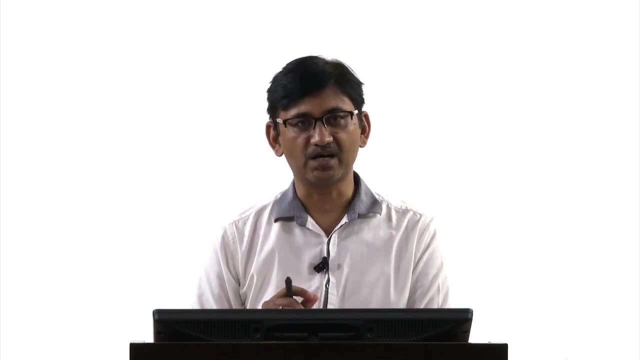 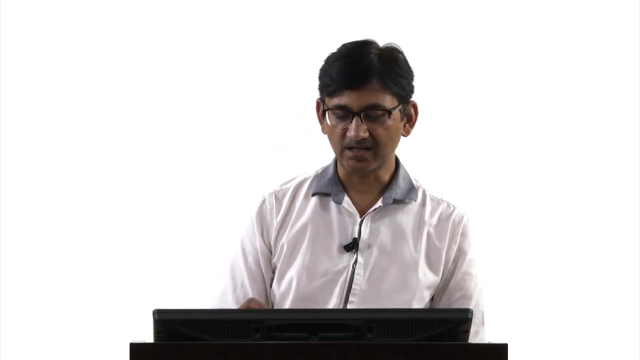 valence band to the conduction band. It leaves behind one hole in the valence band. okay, and that hole can be considered as a positively charged particle. okay, and electron is of course a negatively charged particle. So these charge carriers are called intrinsic charge carriers and semiconductors are called. 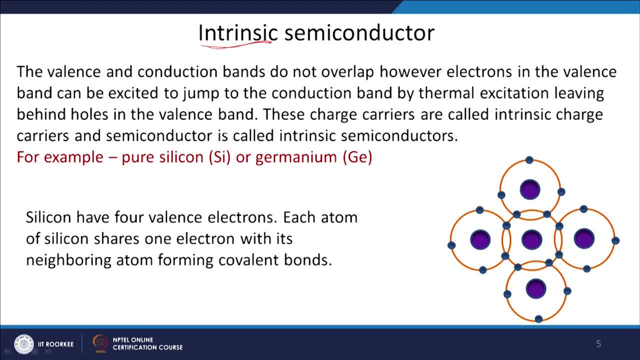 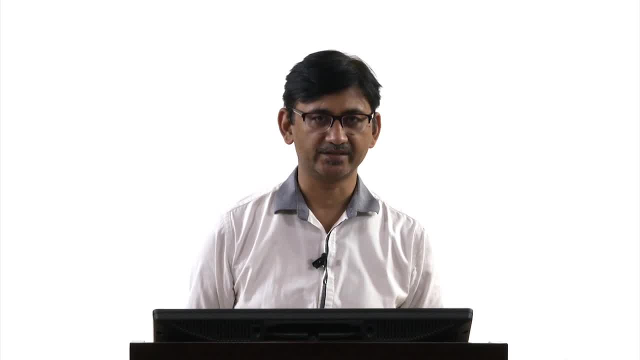 intrinsic semiconductor. so this kind of small conductivity is always going to be there in the semiconductor Because of the thermal excitation. okay, that is why these are called. this is the intrinsic property of the semiconductor. okay, that is why these are called intrinsic semiconductors. 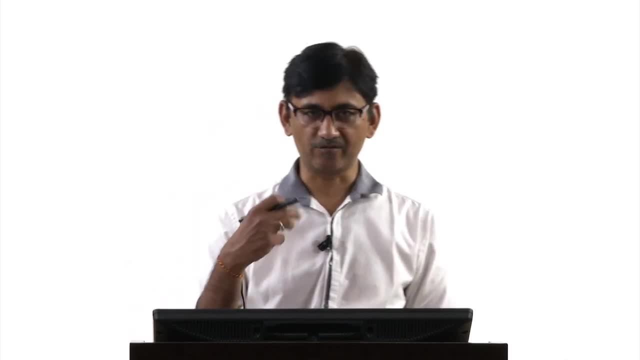 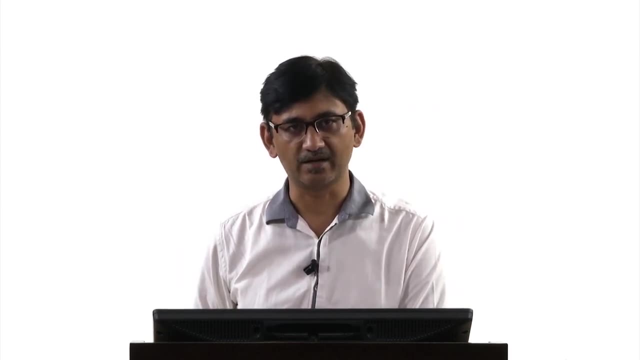 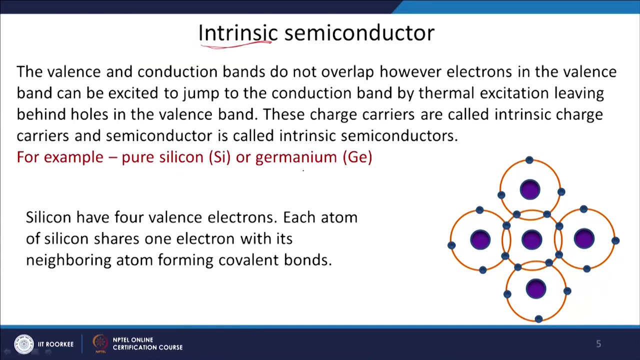 So all semiconductors will have some conductivity. if you are not at 0 Kelvin, okay at any other temperature. there has to be some conductivity in semiconductor and in this condition it is called intrinsic semiconductor. so for example, pure silicon or pure germanium will 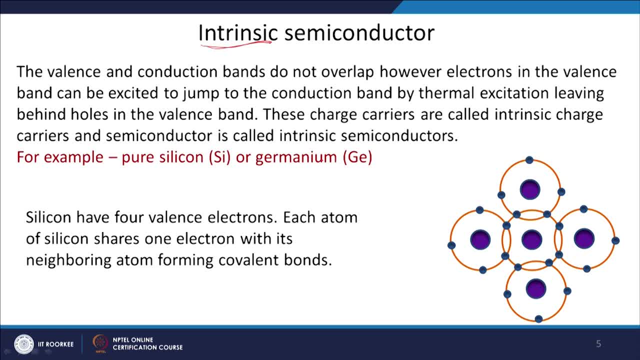 be of this type. okay, of intrinsic semiconductor type, Why they show this kind of property? okay, that silicon have 4 valence electron. okay, basically, here it is shown. okay, so one silicon atom is at the centre and 4 are around. 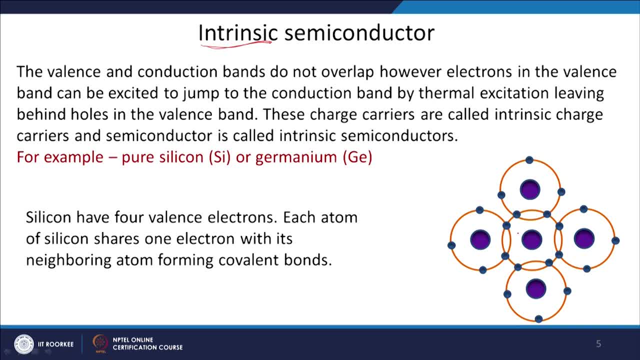 it and they are sharing their valence electrons to fill the fill their outer orbit. so please remember that. So I am not showing the full atomic structure of silicon here, I am just showing the outer orbit here. there will be 2 more orbits in this, okay, which I am not showing it, right? 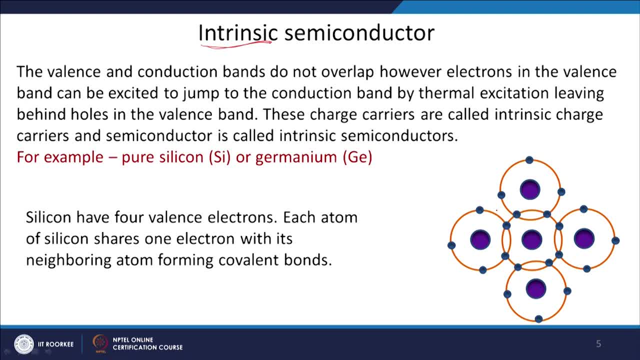 now, because it will complicate the whole schematic here. So only I am showing the outer valence shell, okay, where the valence electrons are orbiting. so one silicon atom in the centre is sharing electrons with the 4. Because in the outer shell it has only 4 electrons. it need 8 electrons to be stable. that is. 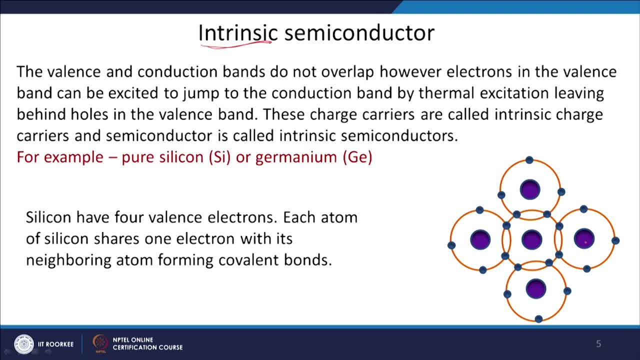 why it is sharing with 4 other silicon atoms. okay, 1 electron to fill its shell with the 8 electrons and may become stable. so with this silicon atom, another 4 will come here. okay, and like that it will be a sharing of electron and covalent bonding will be there. 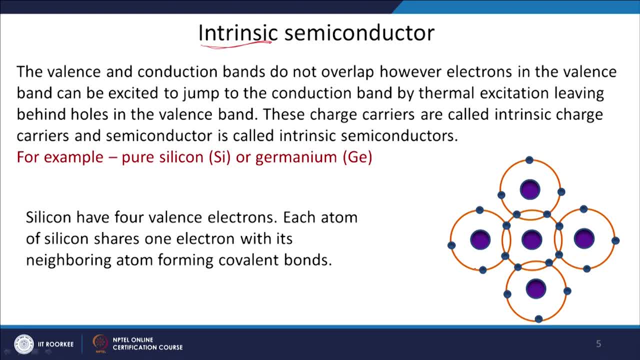 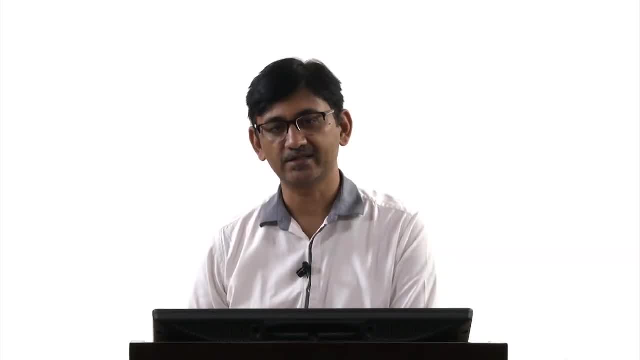 between the silicon atoms. So in normal conditions, okay, Okay. So in normal conditions, you will see that there is not going to be any free electron available for conduction. okay, but as the temperature increases, what happens that this electron may get sufficient energy? okay, to jump from this valence shell and leave. 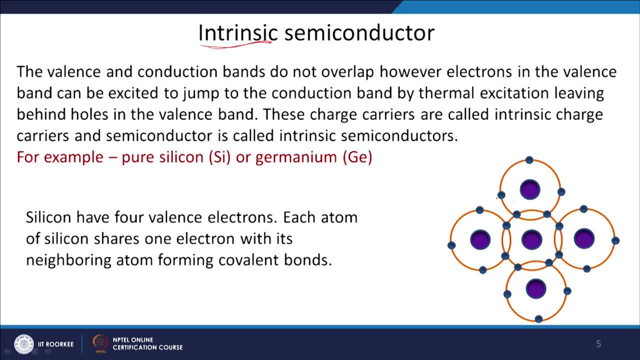 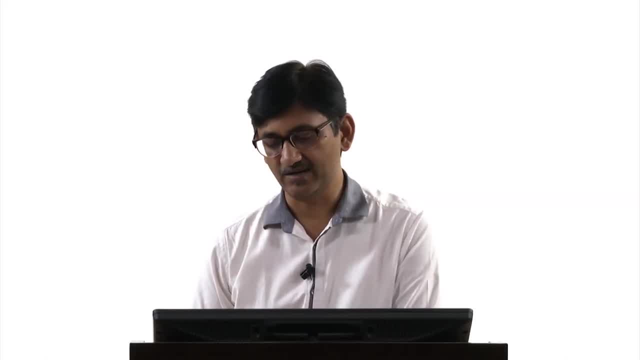 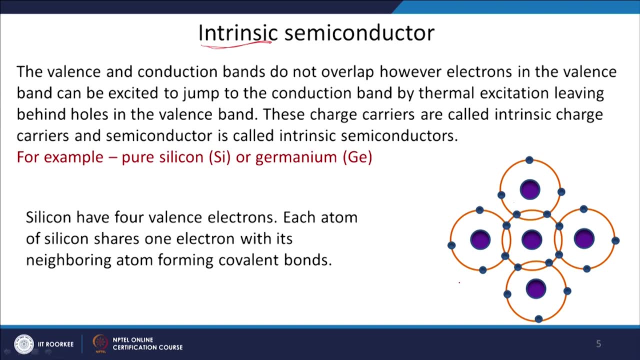 behind a hole here and become free. okay, to carry a charge when electric field is applied, so it can move when an electric field is applied. Okay, So because of thermal excitation it can jump from this shell and go out okay. 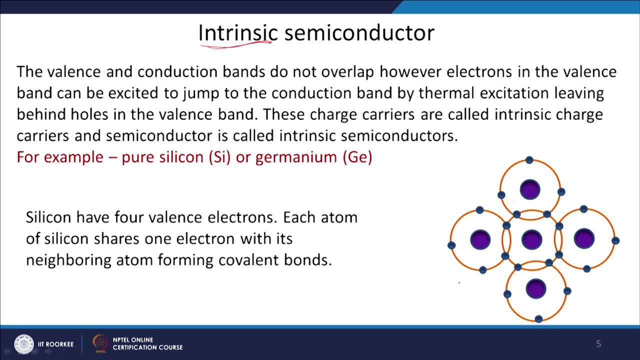 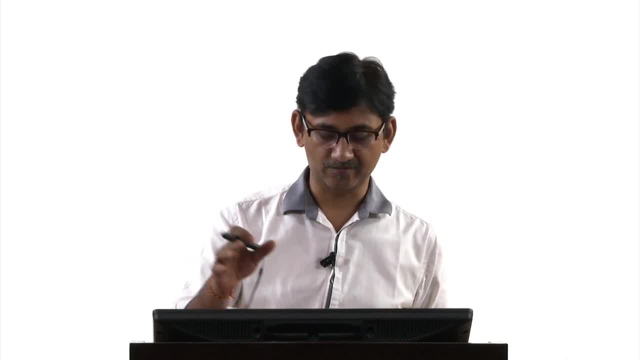 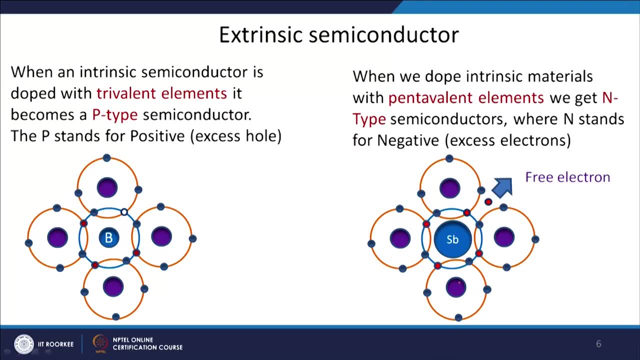 So this is how the silicon arrangement is there, okay, and in this case, when thermal excitation there, there has to be, some intrinsic flow of charge will be there. The extrinsic semiconductor are the ones where you add deliberately some doping agent. so 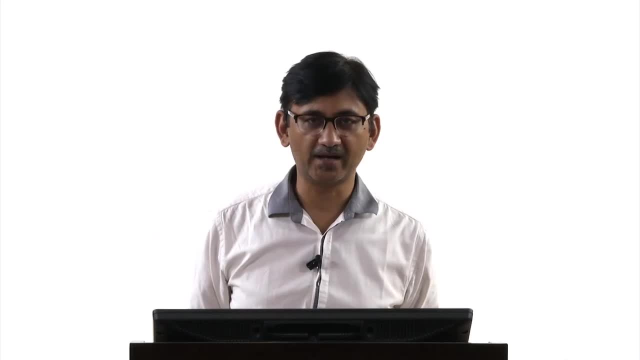 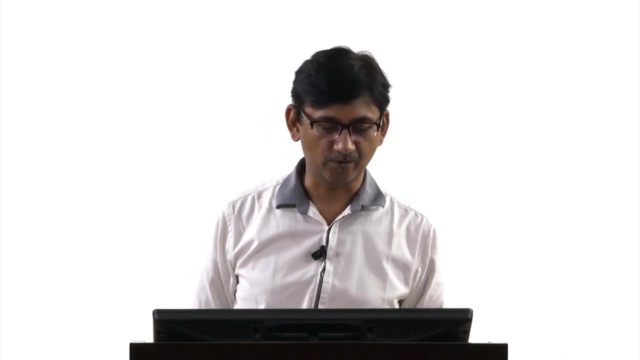 okay, Okay, Okay. So this is what we call as, or doping elements, or this is what we call as doping of semiconductor to add elements of either a trivalent elements or pentavalent. okay, What do we mean by trivalent element? 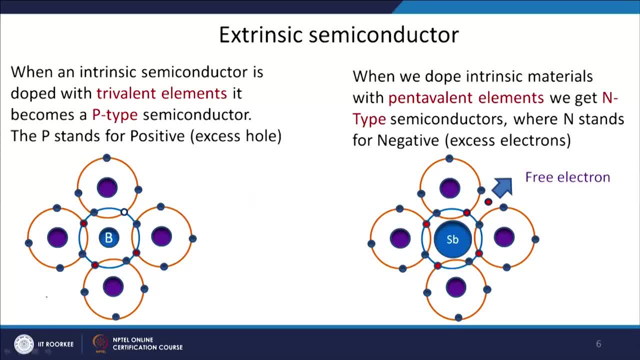 These are the element which has 3 electron in the outer shells. okay, For example, boron here is shown in the centre. okay, It has these 3.. Let us say I will. I think I have shown it by this red colour electrons. these are for. 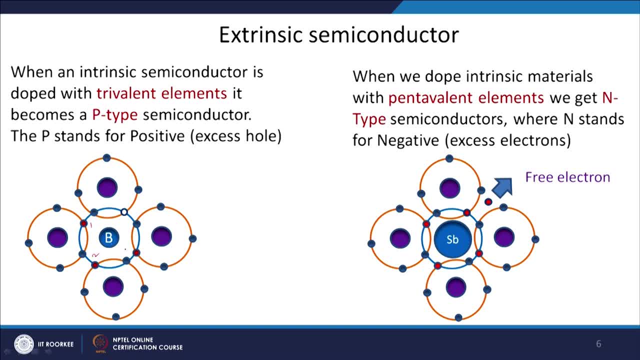 boron. so you have 1, 2 and 3 electrons of in the valence shell of the boron, okay, So these are the 3 valence electrons. so this is a trivalent element, okay, which has 3 electrons. 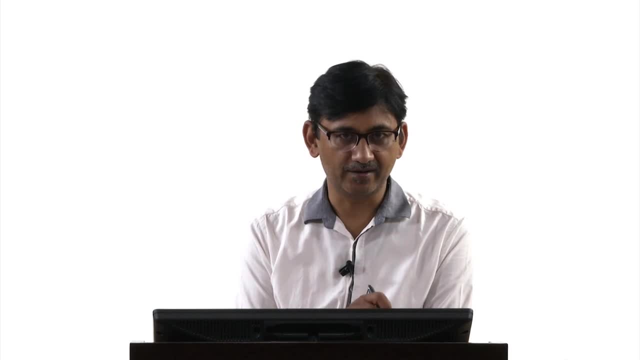 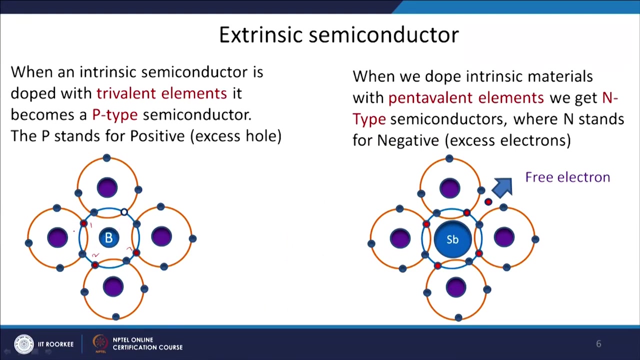 in the outer shell. so when you add this kind of element in the silicon- okay, and this is what we call as doping- Then what will happen is the boron will replace the silicon atom. okay, and now what will happen? earlier, all the silicon atoms were sharing 1, 1 electrons and their shell were getting 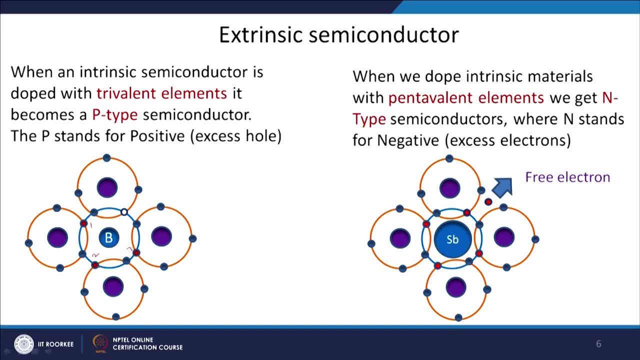 full with all the 8 electrons in the outer shell. okay. But now with the boron, 3 electrons will be shared by these 3 silicon atoms, but with the 4th silicon atom It has no electron to share with, so it is only having a hole present here, okay. 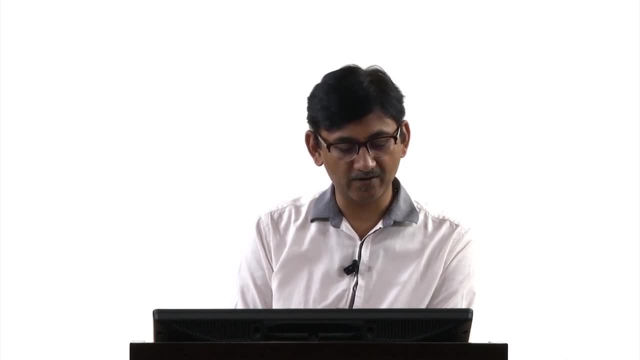 So, with the addition of each boron atom, you will have 1 additional hole present here Now, because it is not sharing any electron. this hole is not bounded by the bonding between the boron and silicon. okay, so it is free to move and as soon as you apply any electric 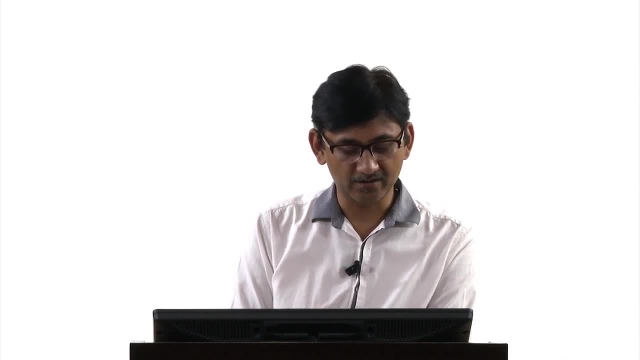 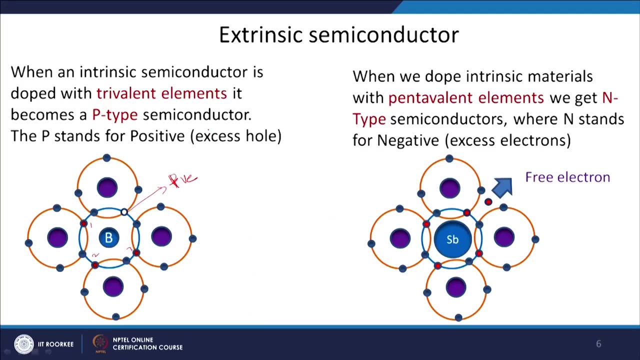 field, this hole will move, Okay, And since hole is considered as positively charged, okay. that is why these type of semiconductors are p-type. So if you add a trivalent element in semiconductor or silicon material, okay, you will get a. 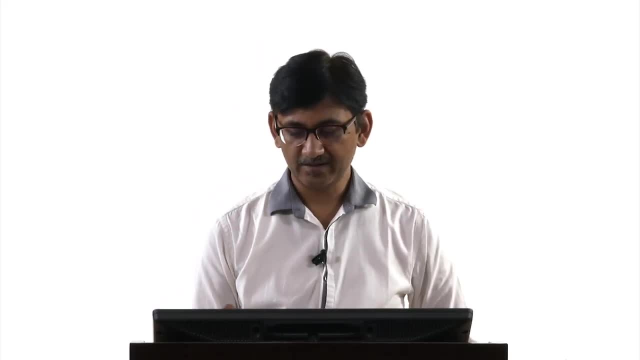 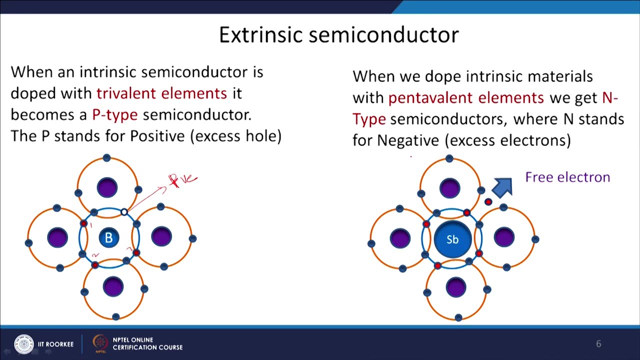 p-type semiconductor. When we dope the same intrinsic semiconductor with a pentavalent element, okay, we get a n-type semiconductor, where n stands for negative excess electrons. okay, So again You can see. antimony is there, okay, which has 5 electron: 1,, 2,, 3,, 4 and 5th one is: 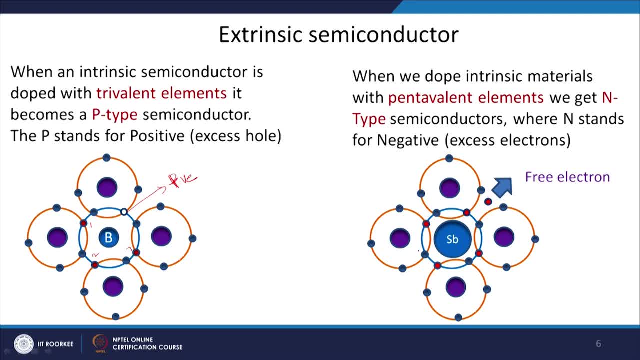 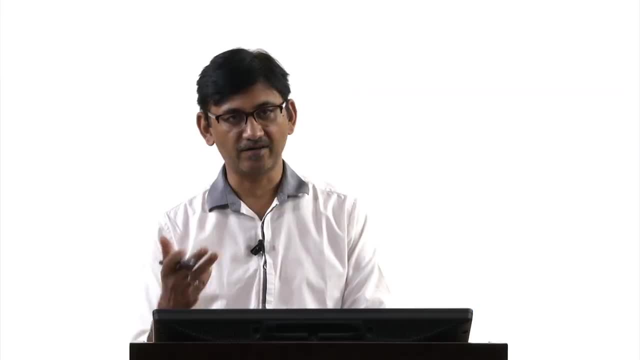 now 1 extra electron is there, So the 4 electrons is shared with the 4 silicon atom around it. 1 extra electron is there which is not shared with any electron, so it is free to move now. So we have increased the conductivity of the semiconductor by adding trivalent element. 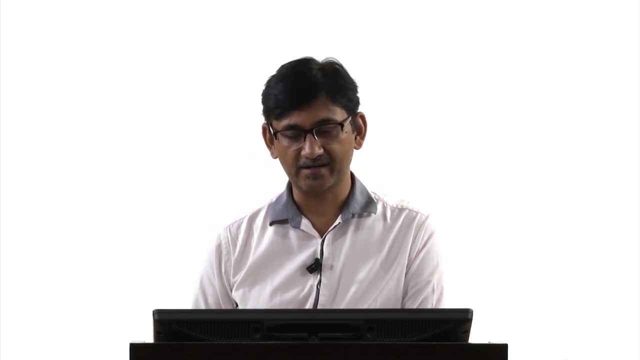 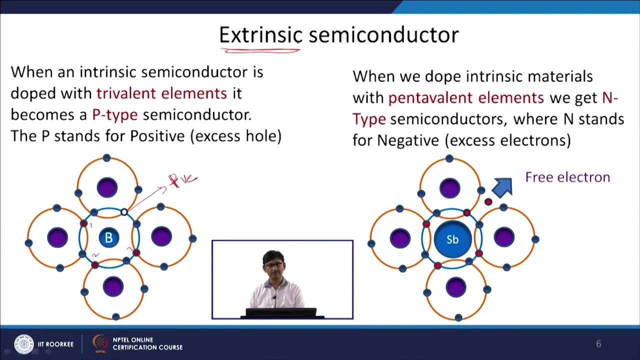 here. okay, And this free electron: when you apply electric field it will be free to move. So these are called extrinsic semiconductor when you add deliberately some element into that to make it either p-type or n-type. So you need both p-type and n-type to make diodes and so on. okay to make a circuit. 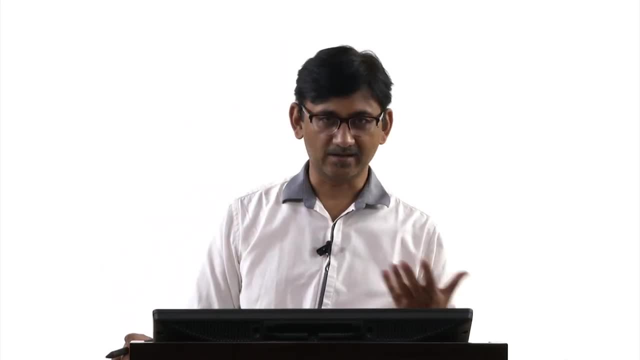 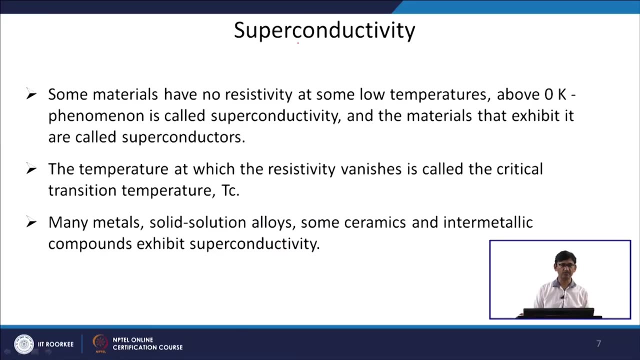 So both are important. Now the superconductivity is another type of property where the material does not show any resistivity to move. Okay To electrical flow. okay, So you can understand for any flow of electricity through normal metallic materials. okay there. 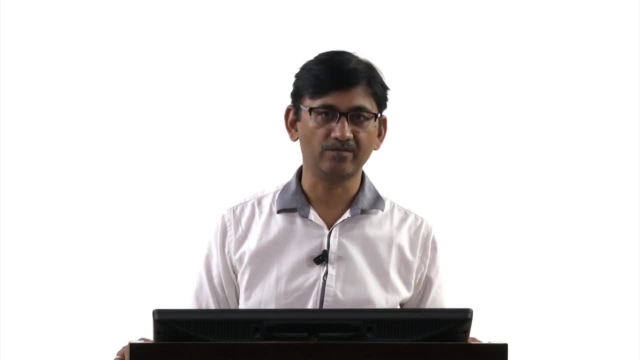 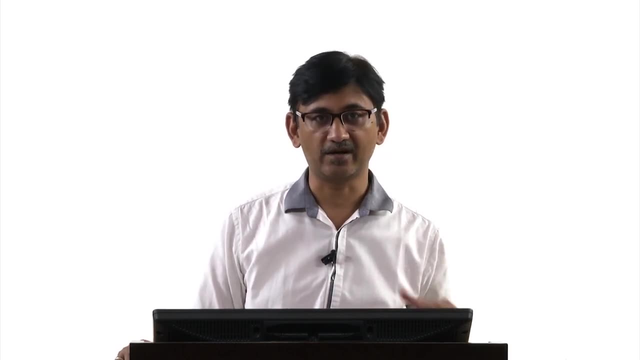 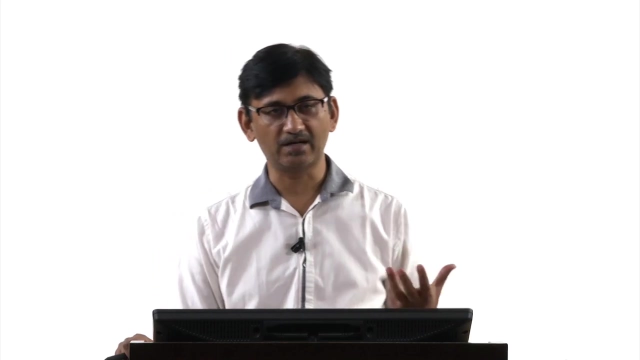 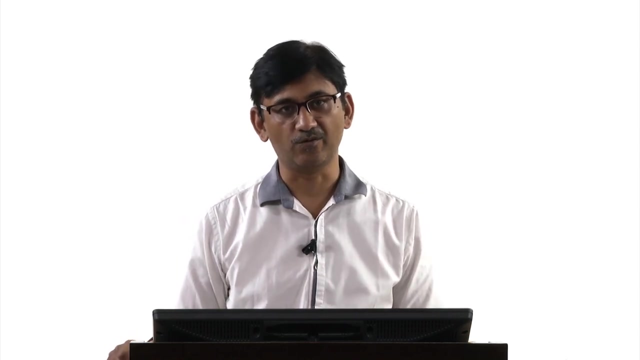 is always some resistance is offered to the flow of electric current, okay, And of course this is significant resistance. okay, And you have significant power loss because of this resistance. So superconductors were when people started thinking about that. So the superconductor does not offer any resistance to electrical flow, okay. 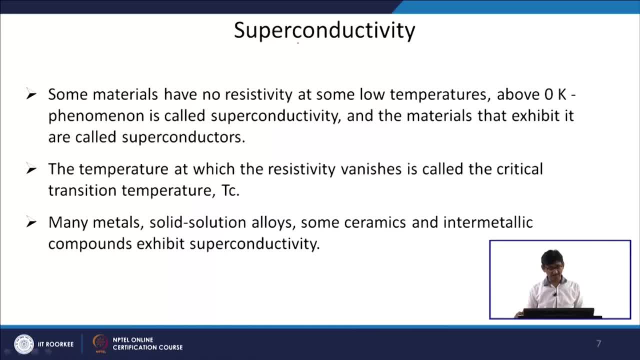 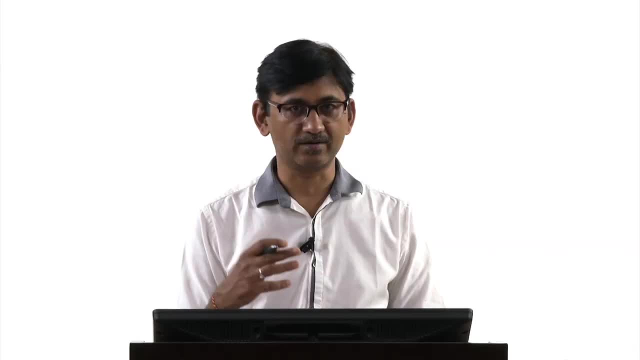 So, and especially ceramics, are some of these type of material which show superconductivity. So these show super, very or nil resistance, okay, at some temperature, But these temperature are usually much lower. so, like at liquid nitrogen and these kind of temperatures, or below that. 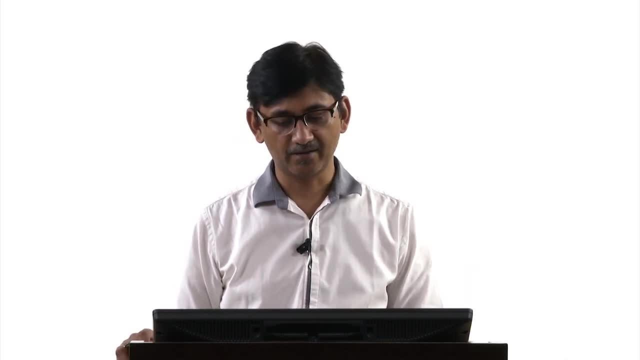 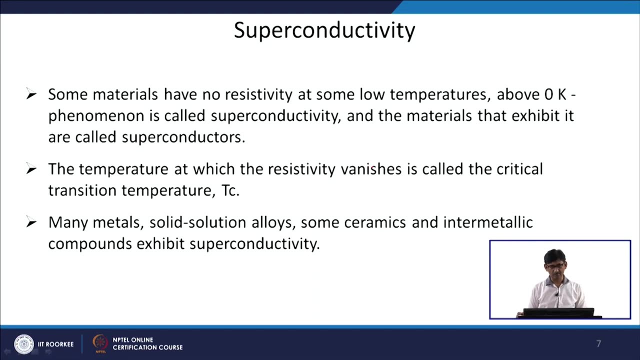 Okay, And they show superconductivity: okay. So the resistivity, the temperature at which the resistivity completely become zero, is called the critical transition temperature, Tc. okay. Many metals and ceramics and intermetallic show this kind of properties- very important. 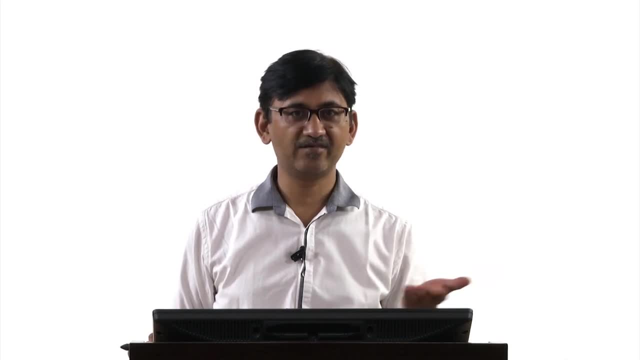 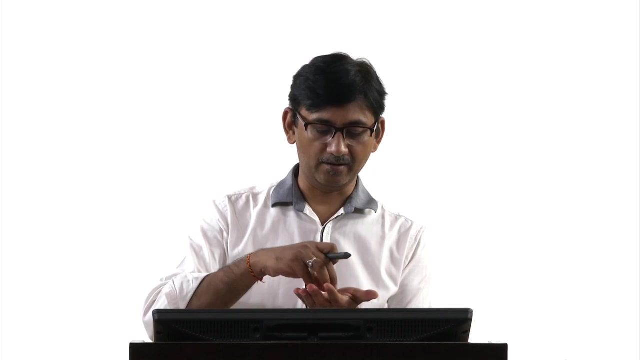 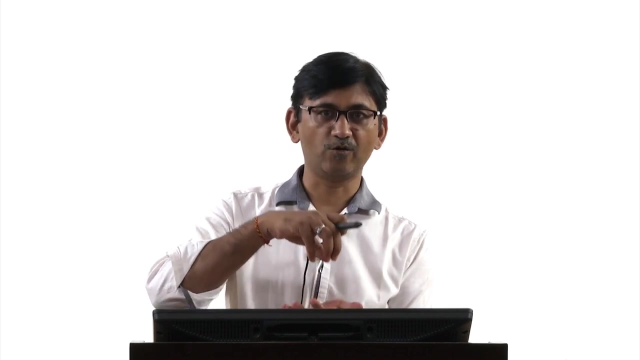 and this kind of Megalev high speed trains. you must have heard of these. Okay, They operate on this principle, okay, That when you have superconductor and you put another conducting metal over that, then it will kind of float over that. okay, 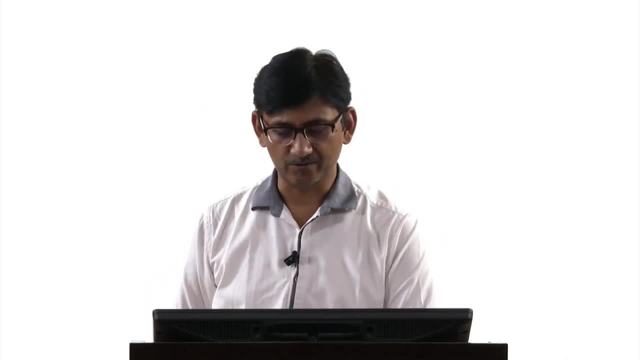 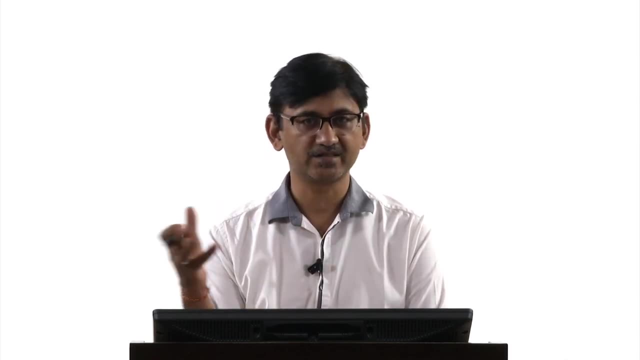 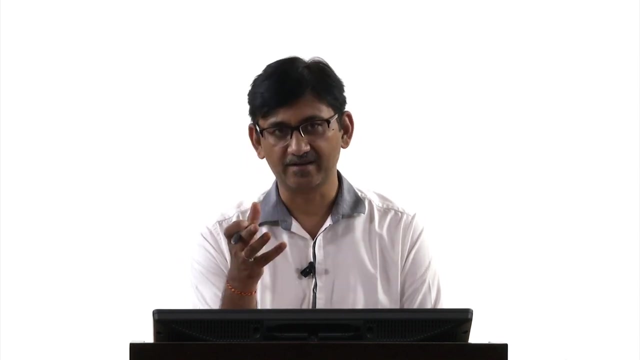 There are lot of theories about that. okay, We are not going into details of that, but these are some important class of materials. now, to have zero friction: Okay, There is no friction movement of, for example, in this case, trains. okay, by having a superconductivity. 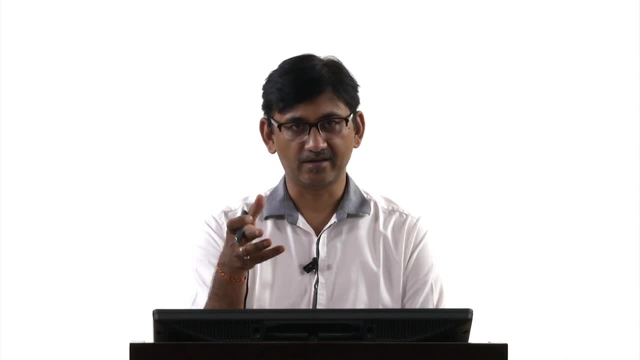 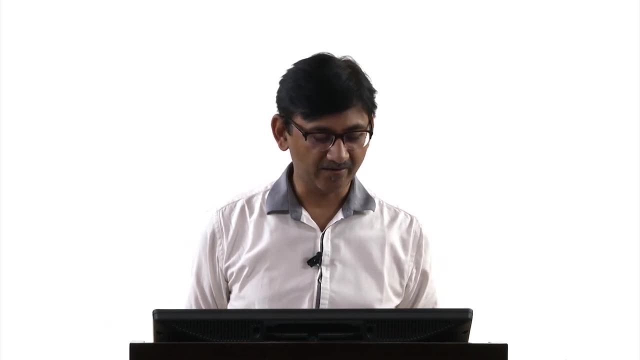 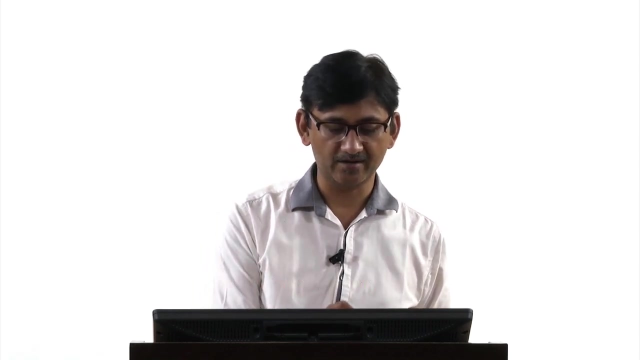 in the, in the where the wheels are there. okay, Then, coming to magnetic properties, the magnetism can be divided into different classes. okay. Dimagnetism is a very weak magnetism which exist in the presence of an external field. 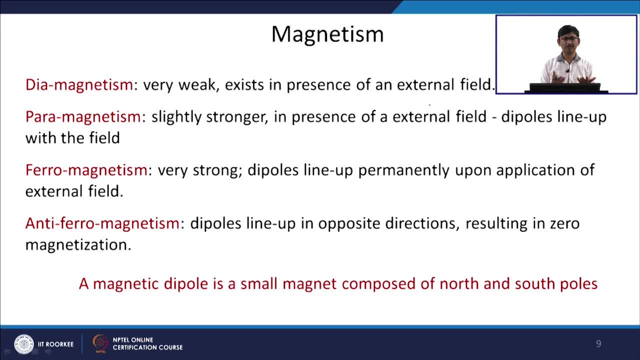 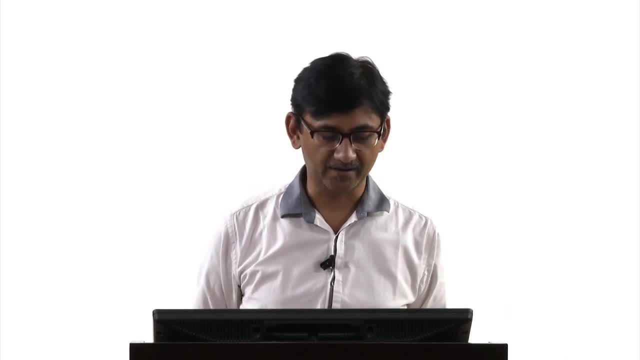 okay, So when you apply the external field only, then you will see magnetism in the material, and when you remove the external field then there will not be any magnetism. Then there can be paramagnetism slightly stronger than diamagnetism, okay. 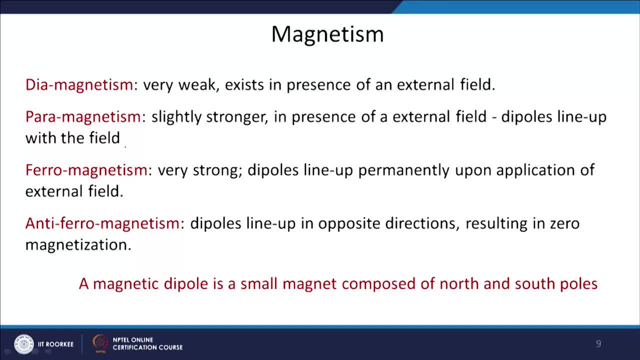 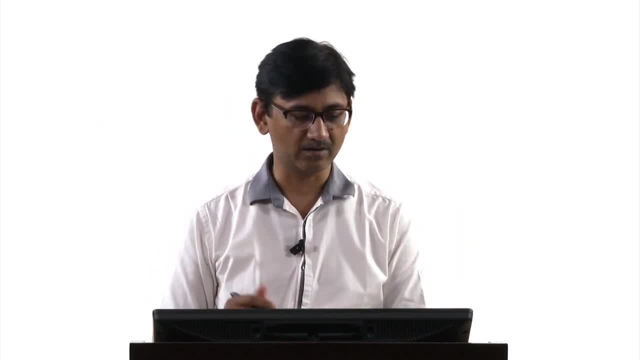 In presence of external field, dipoles line up with the field. so, again, in the presence of external field, you will see some magnetism. it will be slightly stronger than diamagnetism. Ferromagnetism is the one which you usually see. 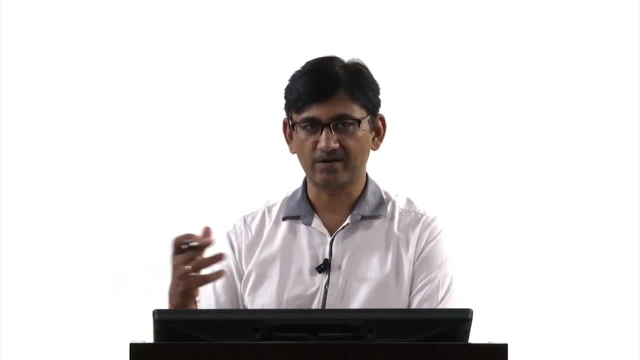 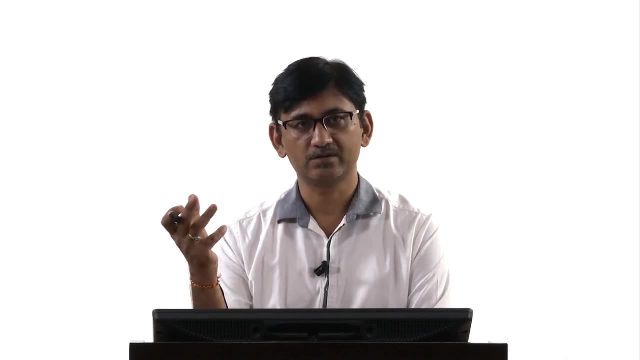 Okay, Ferromagnetism is the one which you usually see in magnets. whatever you use in your, for example, in your music box, okay, there will be some magnetism, they are going to be there. okay, and lot of, for example, your fridge magnet, you will have a magnet. so 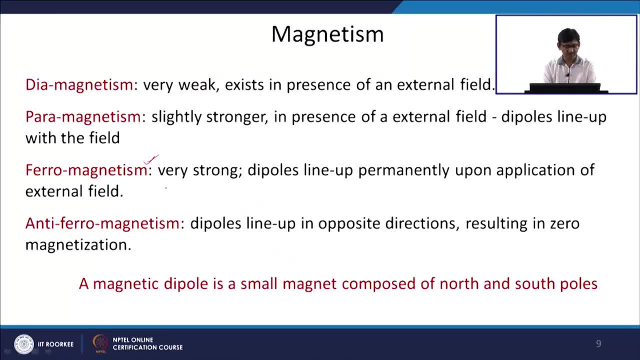 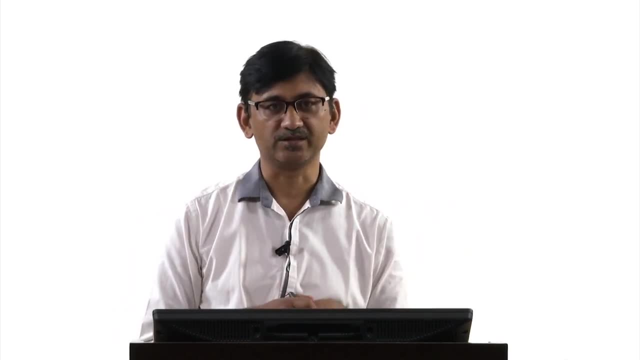 all these magnet are show ferromagnetism, which is very strong magnetism. they show because the dipoles line up permanently Okay, Upon application of external field. so when you apply the external field, okay, they permanently show magnetism. so ferromagnetism will always show magnetism once you have induced the magnetism. 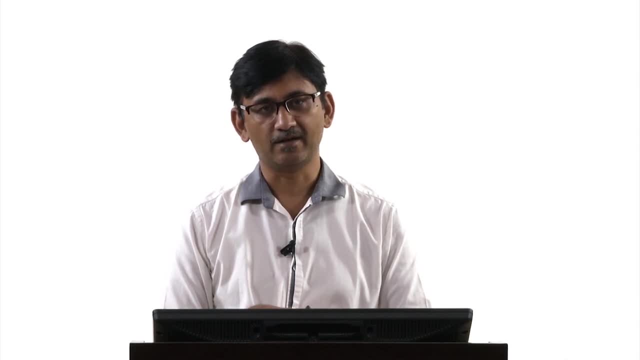 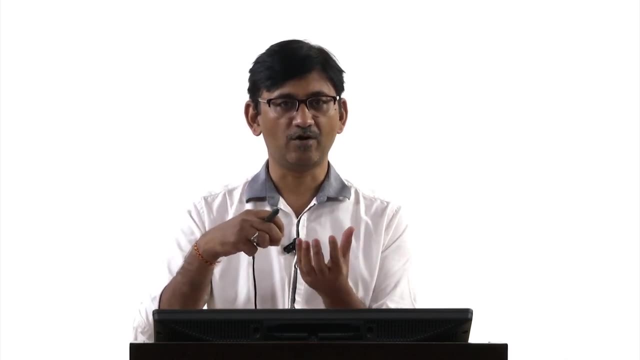 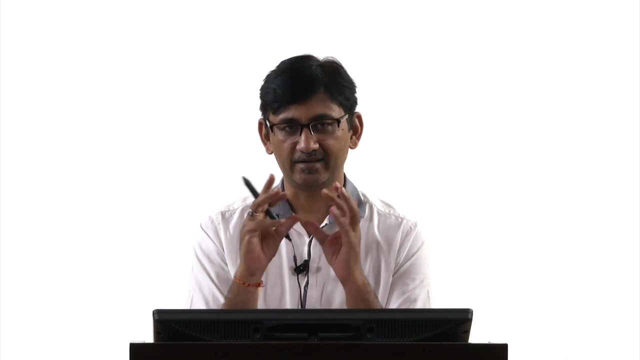 in that, in that particular material For example, if you might have seen, there are some time on the office table, some jar is there to store the pins, all pins, Okay, Okay, And there is a magnet around it, then the all pin also start showing magnetism. after. 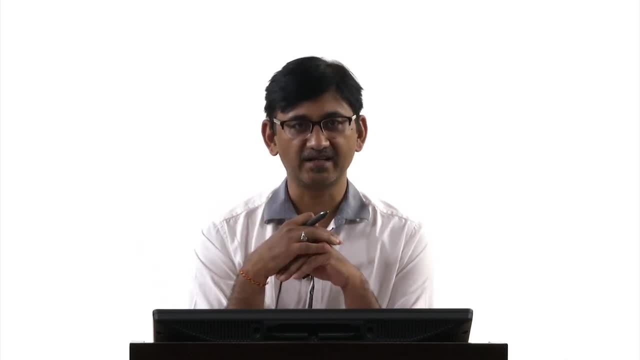 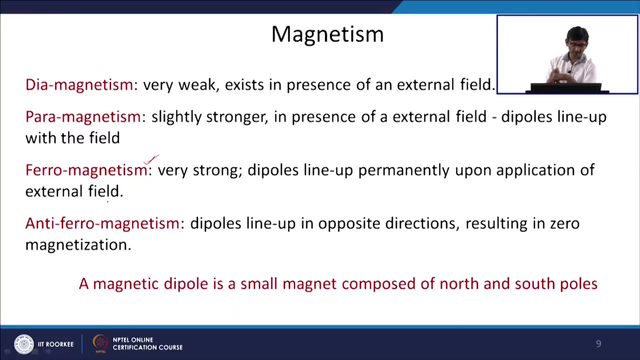 some time. Okay, So under an external field they get magnetized and they remain magnetic even after removal of the external field. Then anti-ferromagnetism is: are there? okay, so dipoles line up in opposite direction, resulting in zero magnetization. so in this case you, if you apply the external field, also you will. 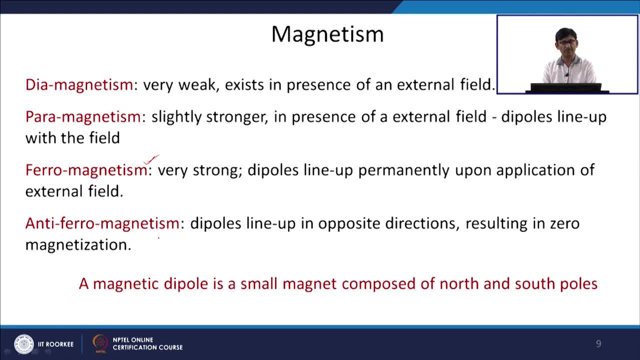 not get any magnetism, okay. so these are anti-ferromagnetism, so anti of magnetism, So anti of what we have discussed just now. a magnetic dipole is a small magnet composed of north and south poles. okay, 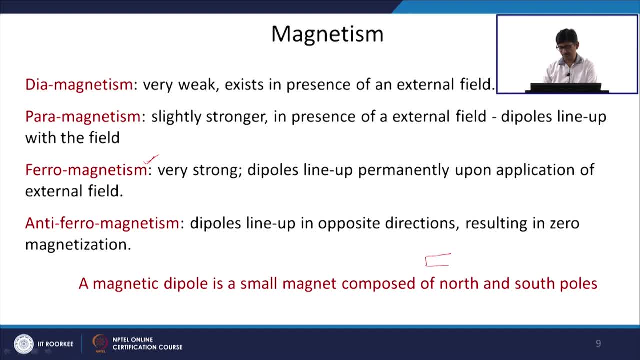 So basically, for any magnet, we have already seen that you will always going to have some south and north pole, okay. so when we say magnetic dipole, okay, basically we are talking about an arrangement where they are arranged in this fashion: south and north. so if all, 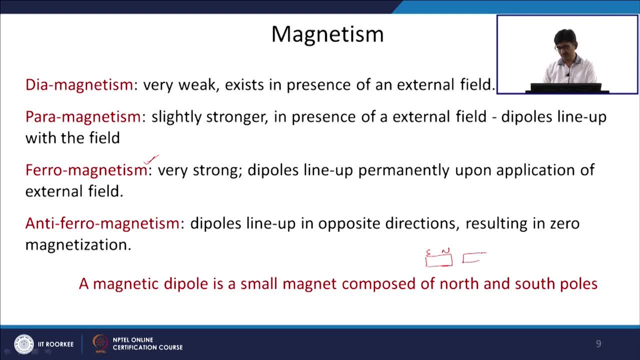 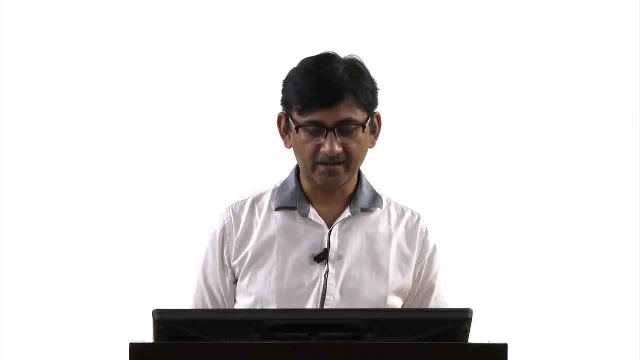 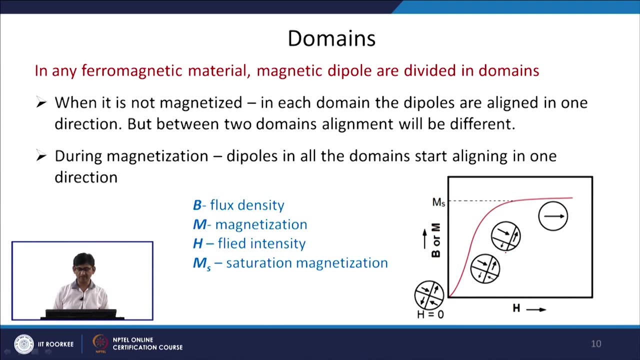 the dipoles are arranged in the same fashion. okay, Then you will have magnetism. okay, So in any ferromagnetic material- we will now consider basically ferromagnetic materials, only here- okay, magnetic dipoles are divided into domains, okay, so if you take any material, 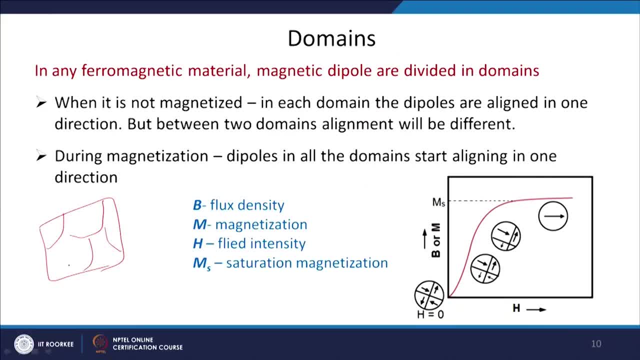 they will be. there will be some domains will be there, okay, like grain boundaries or grains. okay in material, Where the In one domain the dipole will have one type of alignment, okay. in another domain they may have a different alignment. for example, okay again, those dipole, north south dipoles. 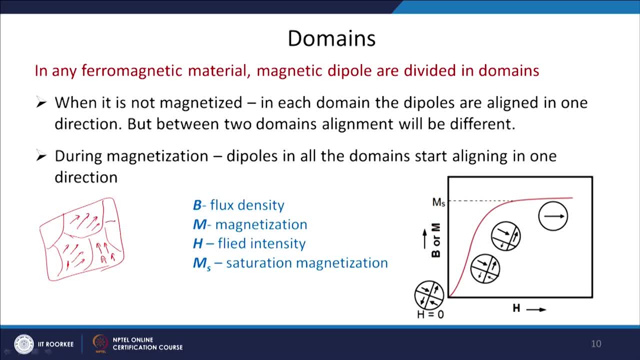 and maybe another domain. they will have another alignment and so on. okay, These are not grain boundary, these are domain boundary. so one domain can consist of, so this can be, So a domain can be within one grain, so you can have one grain like that in this one. 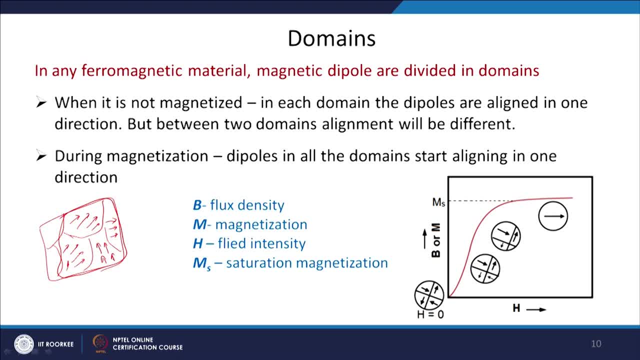 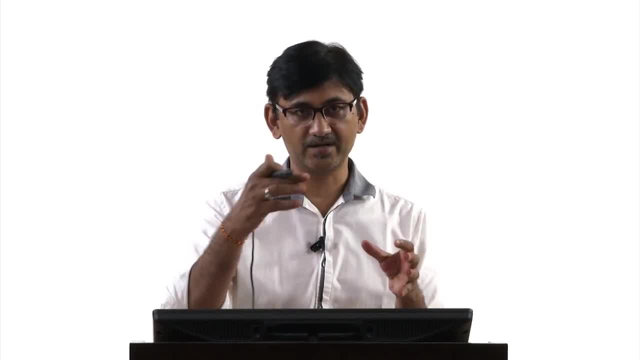 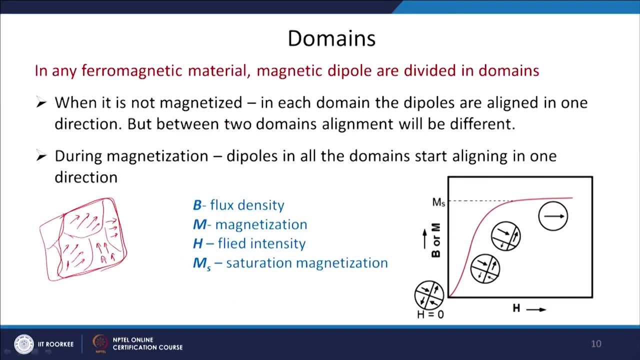 grain. you can have domains like this okay within a grain itself, so they are not divided between the grain. single grain can have multiple domains- okay, and each domain you will have some alignment of dipoles. So when it is not magnetized in each domain the dipoles are aligned in one direction. but 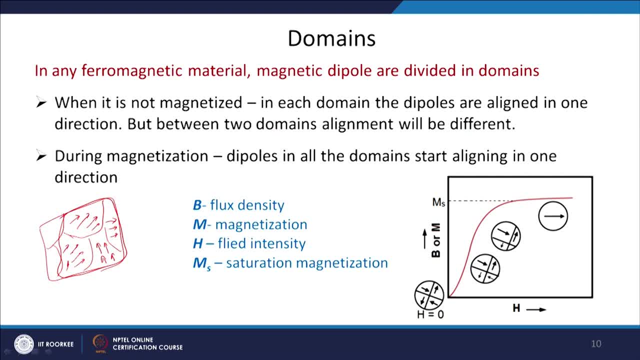 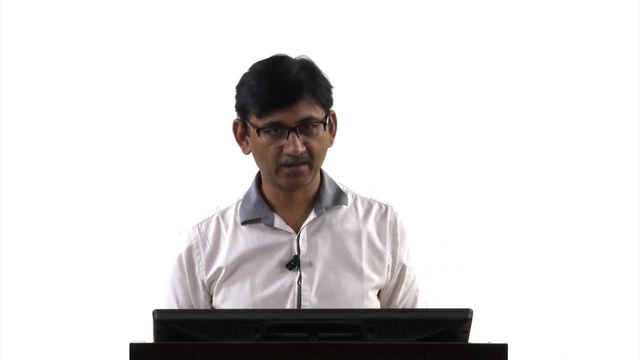 between two domains, alignment will be different. okay, So in a domain the alignment is going to be same, But if you compare between two domains, the alignment is going to be different. so when it is not magnetize in all these domains they are aligned in very random way. okay, but 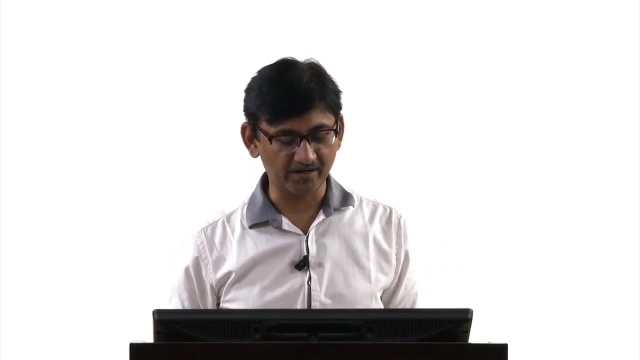 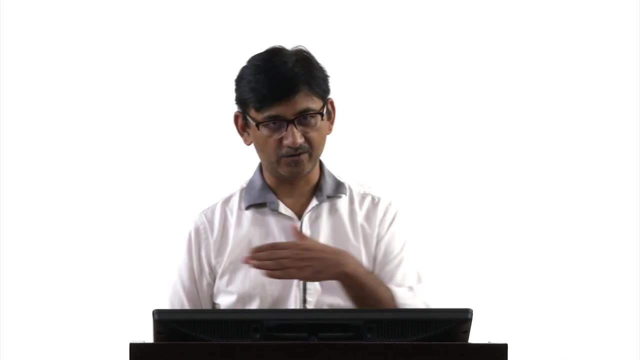 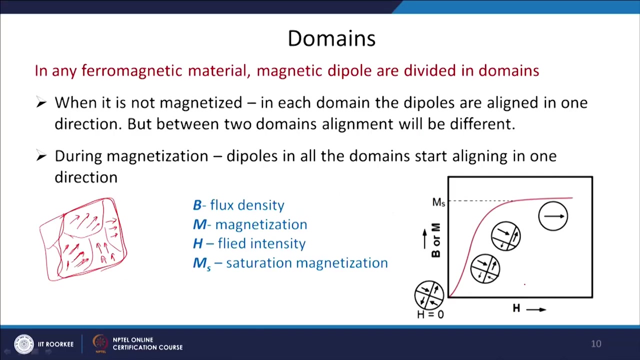 when you do magnetization, okay, during magnetization, dipoles in all the domain start aligning in one direction. okay, so when you do magnetization, all these domains will start aligning in one direction. So which can be shown by a curve like this, where it is called a BH curve, where B is your. 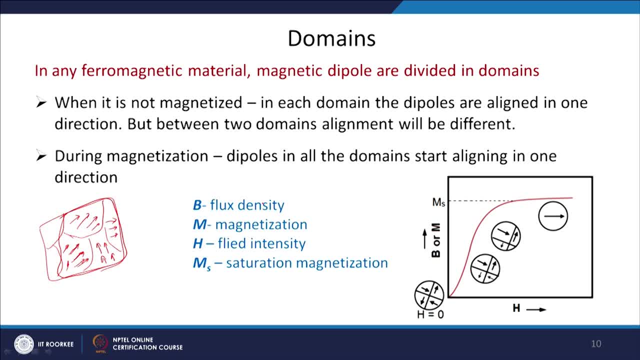 flux density, which is we are inducing the magnetic flux density in the material, M, or you can say M also magnetization. H is the field intensity. I am sorry there is spelling is wrong here. So field intensity is there H. okay, on the x axis. so this is what, externally, we are applying. 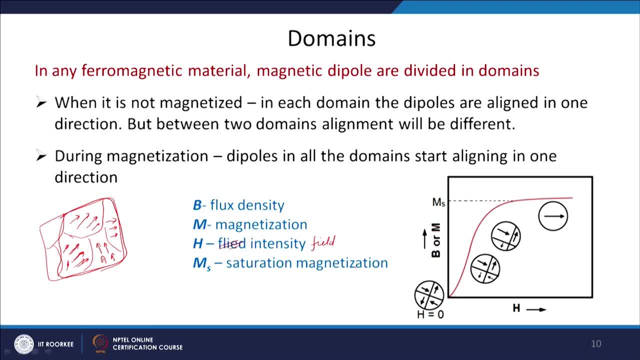 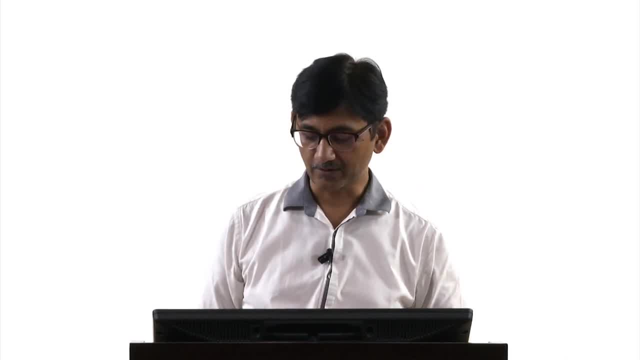 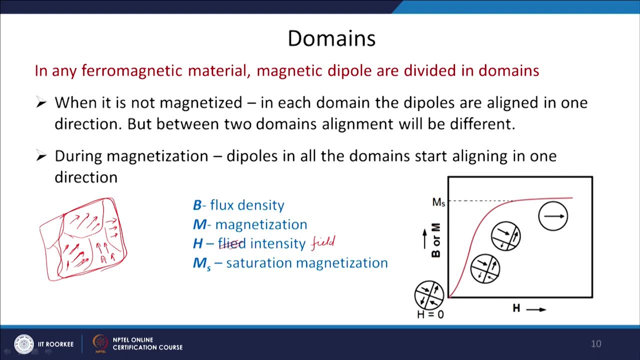 on the material and MS is the saturation magnetization. okay, so what happens when you start applying a magnetic field on a material? okay, so initially they have these domains and alignment of dipoles will be different in each domain, and you started applying some magnetic field on this material. 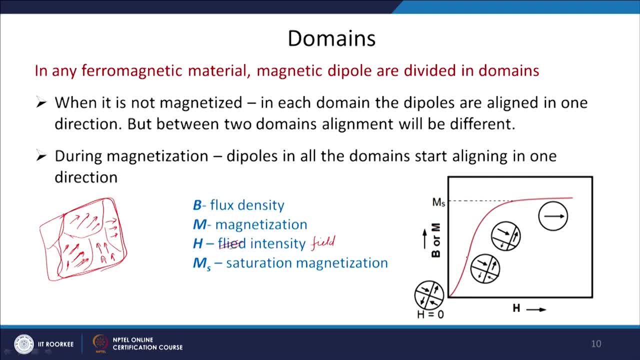 for magnetization. Okay, What will happen? that slowly the flux density, the magnetic flux density, will increase in the material as a function of H, the external applied field intensity. so you can see that slowly the domains are started changing. so some domains are disappearing. okay, and as 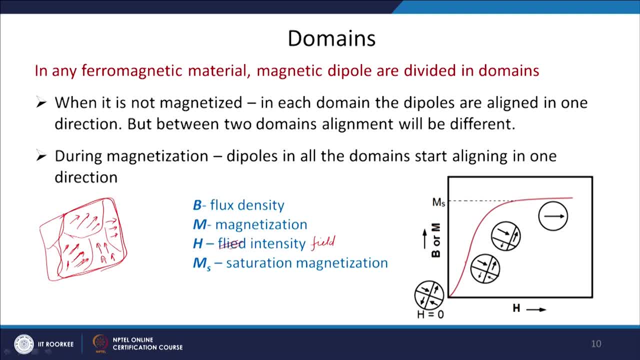 the H is increasing, B is increasing. you reach a saturation point when all the domains are disappeared and, throughout the material, you have only one alignment of dipole, which is in this direction. okay, so, as I told you, all the in all the case, the alignment is same. 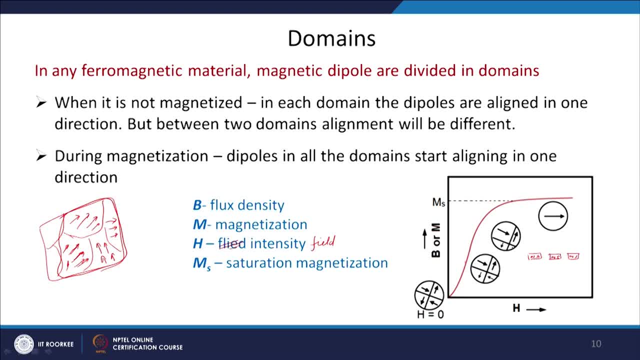 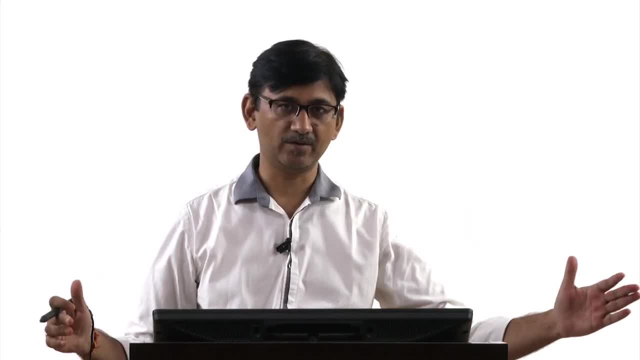 north, south, north, south, north, south, and so on. okay, so now when all the alignment of the dipoles is in the same direction, so one end will be a south pole, another end will be a north pole, okay, and you will have a magnetization in the material. so when the whole material 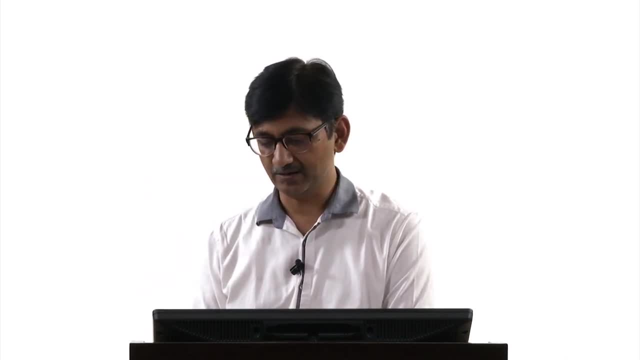 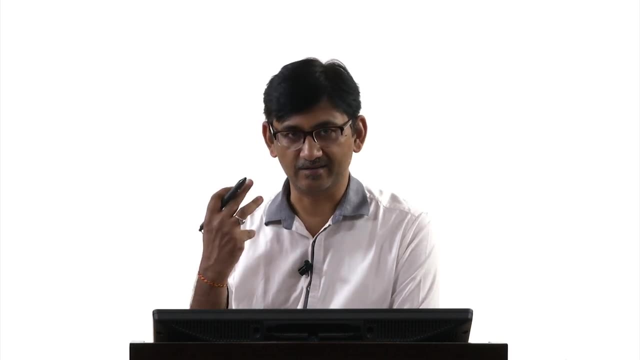 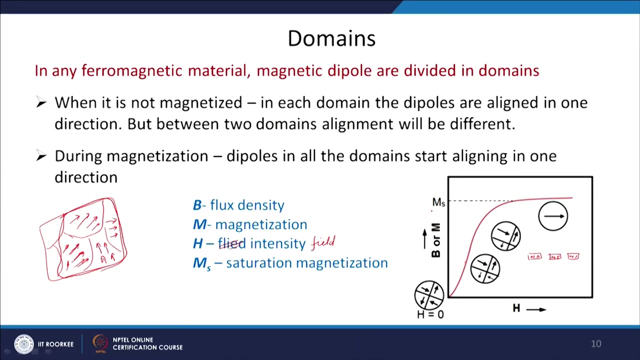 is of one alignment, then you have reached the saturation. now you cannot do anything else. okay, you can keep increasing the external field, but you cannot go beyond that. all the dipoles are in one alignment, so you have reached the saturation point. so this is my saturation. 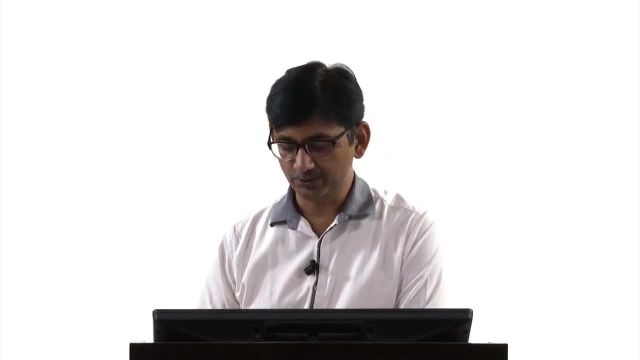 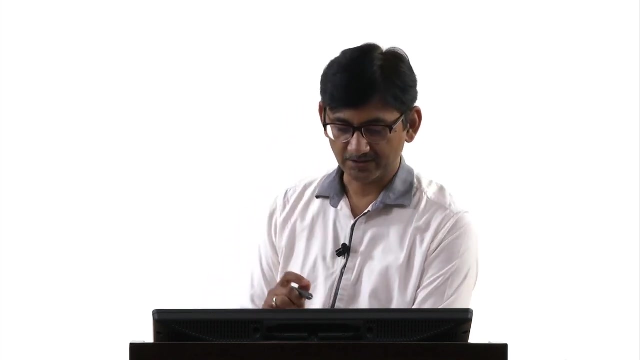 magnetization. okay. Now, once you do that, what happens when you again bring down the magnetic field? okay, that is of interest For us because that actually bring about phenomena called hysteresis. okay, and that is important for our material application. so the hysteresis, what do we mean by hysteresis? okay, so when? 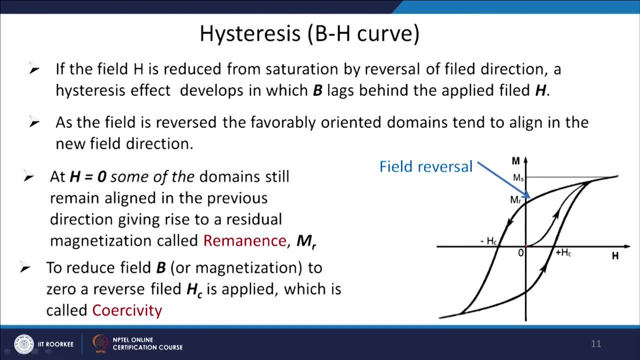 you start the from this point. okay, when the material was not magnetized. okay, you applied a external field, The magnetization process. okay, and it reached the saturation magnetization- okay. now you are reversing the field. okay, so suppose you apply a field such that a given component 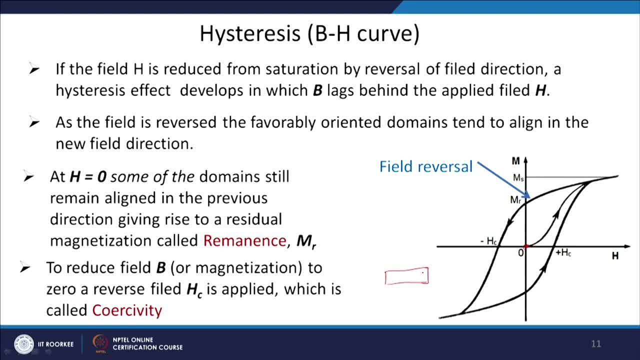 okay, suppose something like this: by applying an external field. now this is what is: the dipoles are aligned such that that you get these two poles in the material and now you have reversed the external field. What will be will happen? that the dipole will again align in the different direction and 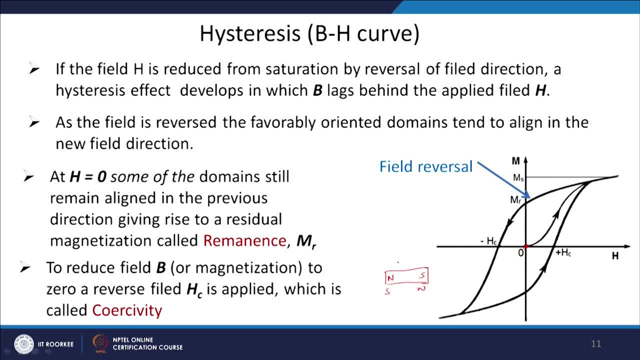 the north has to become south and south has to become north, so all the domains have to align in a in the opposite direction. now, okay, so we are reversing the field now here. okay, so you can see that we started from 0 for external field when the flux density was 0. 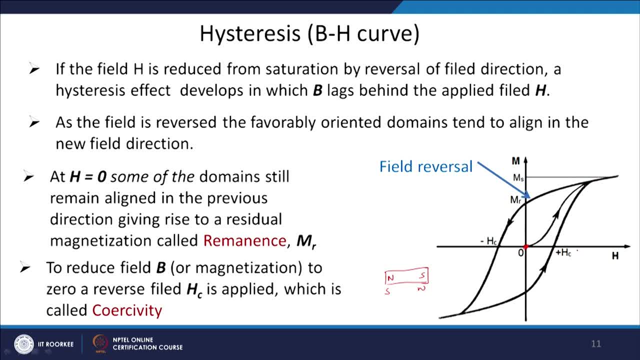 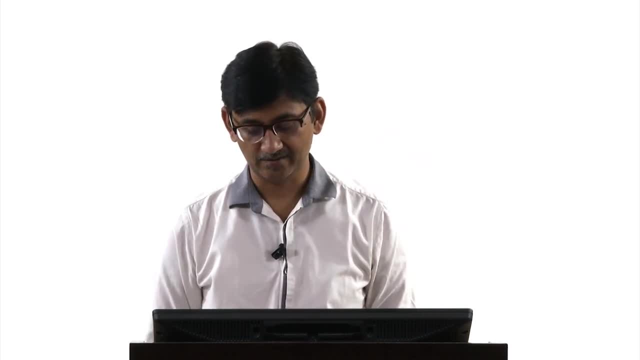 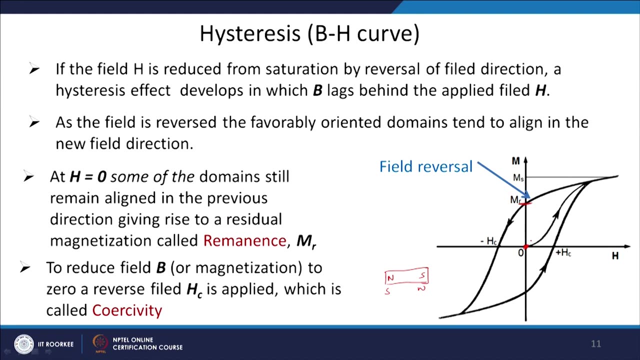 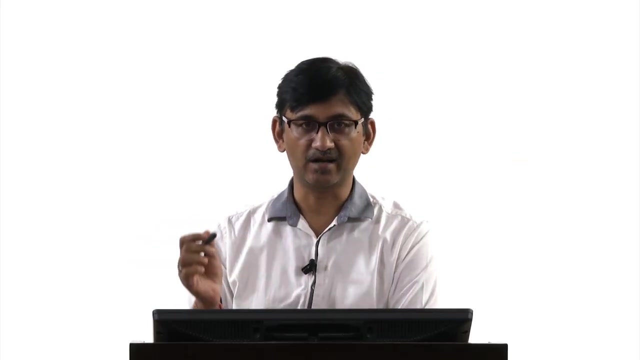 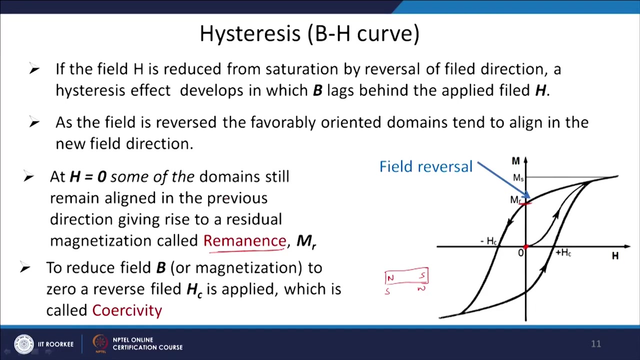 okay, It remained in the in the material because all the domains could not get aligned in the opposite direction when we reverse the field. so while reversing at H is equal to 0, some of the domain still remained aligned in the previous direction, which we did while magnetizing. 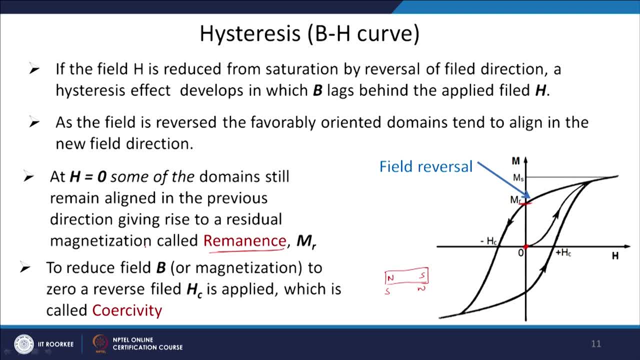 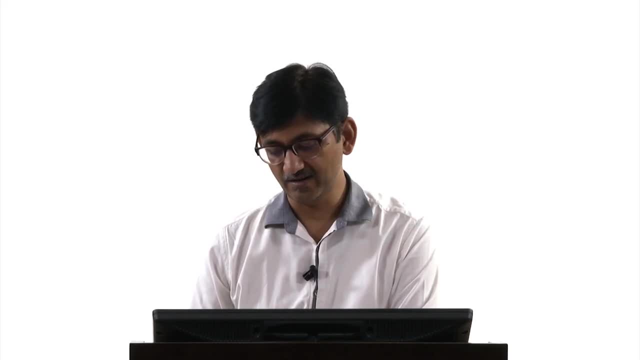 which give rise to a residual magnetization which is called remainance, MR. okay, so that much will remain in the material to get rid of this magnetization. So we have to now go into the negative direction of the electrical field. okay, and this is this. 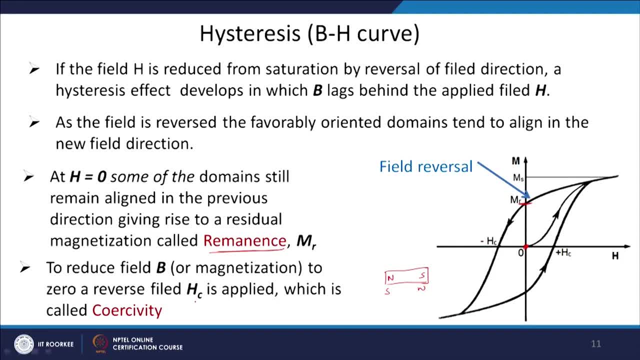 how much negative we have to go will be given by Hc. so to reduce the field B, or magnetization, to a, 0. okay, so now we have come to the 0 flux, the flux density in the material. okay, reverse field of Hc is applied. 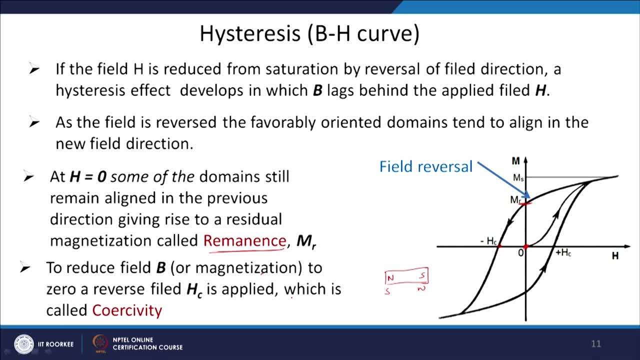 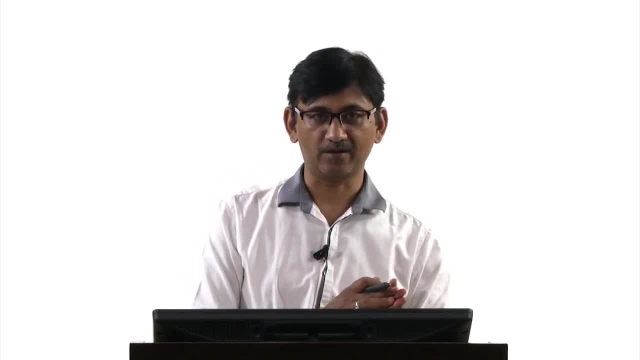 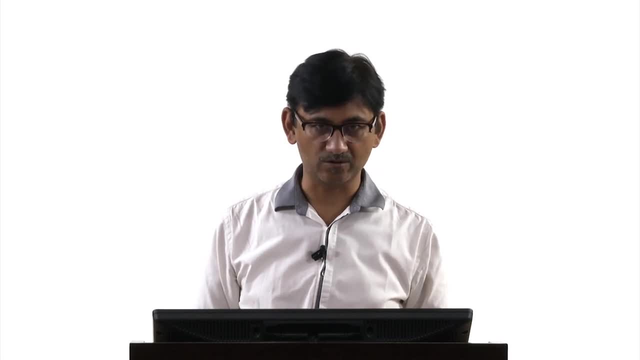 So negative of this external field is applied, which is called coercivity. so, basically, you are coercing the material to bring down the flux density to 0. okay, so you are, you are forcing the material. okay, so, because you are coercing it, this is called coercivity and 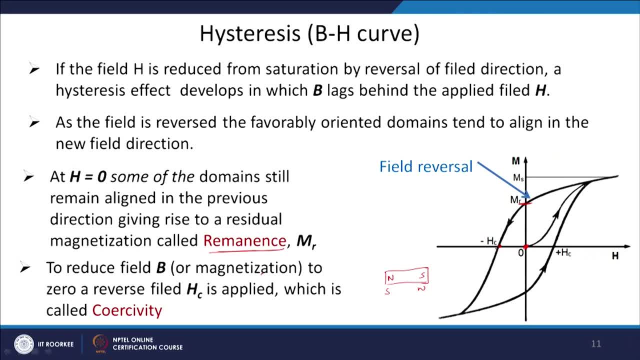 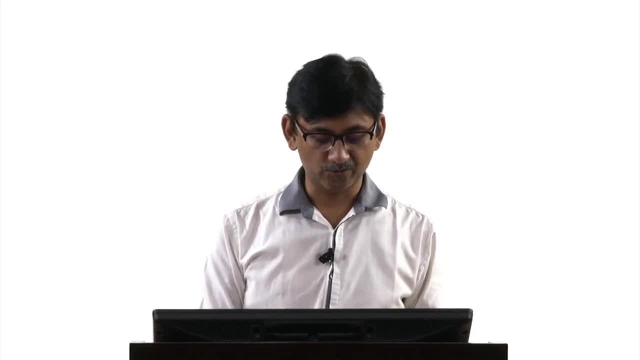 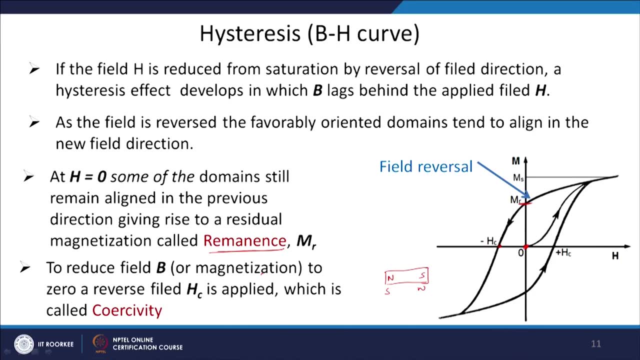 this much negative energy, negative external field you have to apply to bring it down to the earlier state from where we started. So this is the important properties of any magnetic material: that what is the remainance value and what is the coercivity value? okay, and this happens during the field reversal. 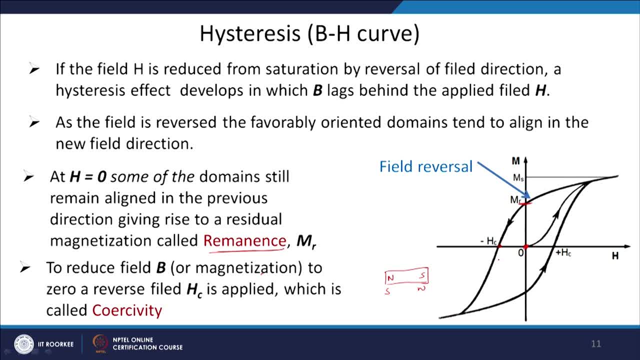 so again you can go into the negative direction as you went into the positive direction. here, again you will reach a saturation. now the whole, all the domains, are reversed and they are aligned in the reverse direction. So again you will reach a saturation point. okay, and when again you start applying reversing, 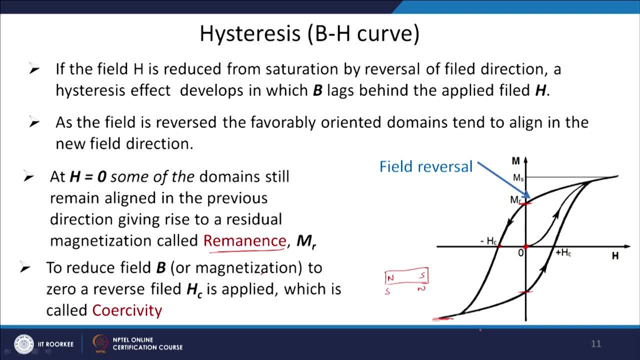 the field. So you will see that some remainance field will be there, some coercivity will be there. that means some positive external field has to be applied to bring it to 0 flux density again and then it will go back to the saturation. okay, so you can see that in each of this cycle. 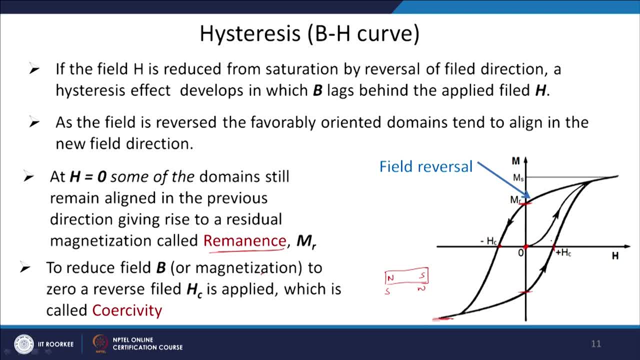 okay, you are losing some energy, so there is an energy loss in each of this cycle. okay, Because it is not following the same. if it would have followed the same curve, okay, maybe it would have gone like this, and again, as you reverse the field, it will go like this: 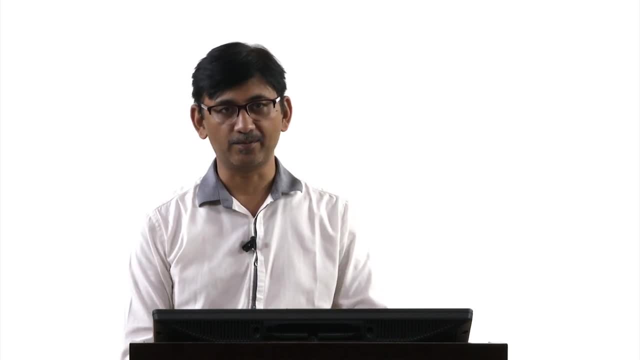 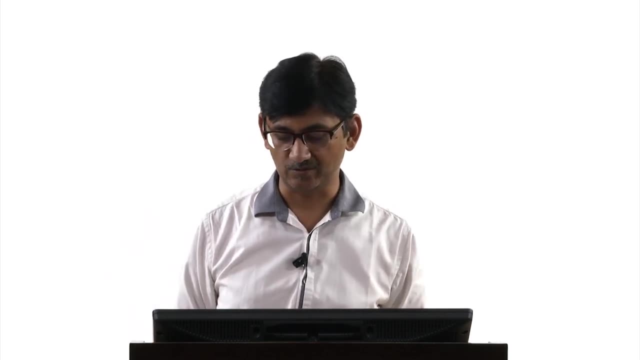 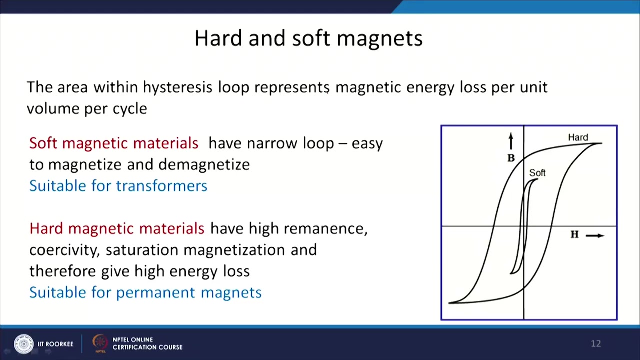 then there would not be any problem, then it would not lose any energy in the this process of magnetization, demagnetization and so on. okay, Now, depending upon this hysteresis loop. okay, so the area within the hysteresis loop represent magnetic energy loss per unit volume per cycle. so in each cycle you lose an energy given. 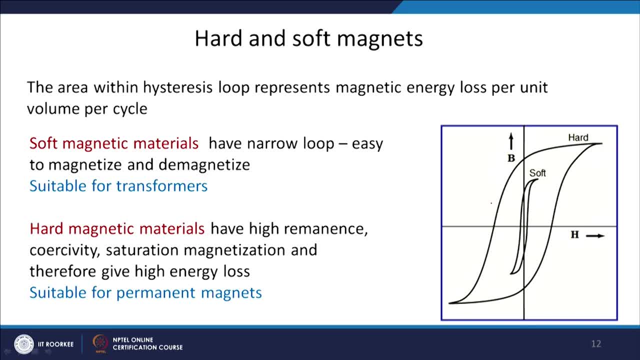 by the area of this loop. okay, because this much extra energy you have to apply to bring it back to 0 and then take it to the negative side, and so on. so in each of this cycle, when you do the magnetization, demagnetization, then go into the negative direction, okay, you lose. 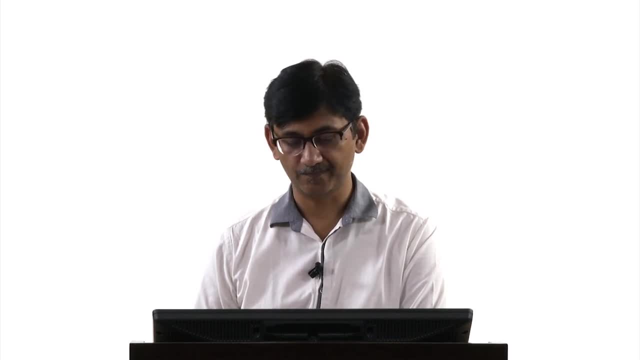 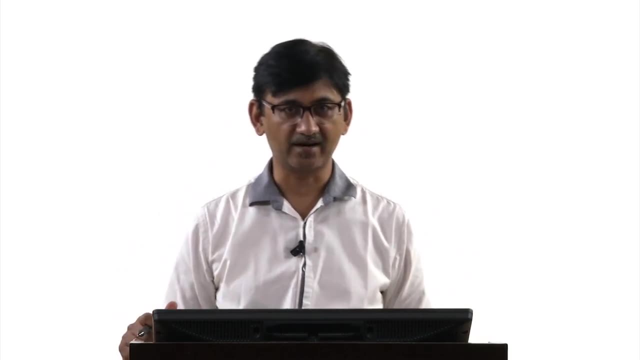 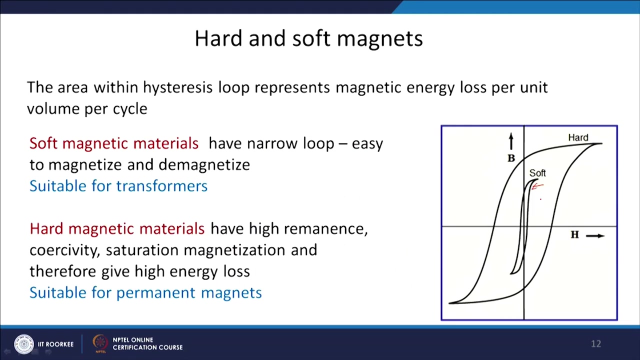 certain amount of energy, Which is equal to the area of this loop. so now, depending upon this area of the loop, I can define two types of material. one is soft magnetic material, another is hard magnetic material. okay, so soft magnetic materials have narrow loop. okay, so this is a soft magnetic. 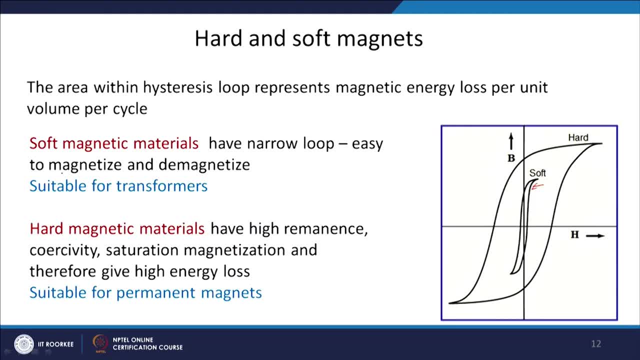 material. that means you can have easy. these are easy to magnetize and demagnetize. I can easily magnetize them and demagnetize them because you will have smaller Remanence, you will have need a smaller coercivity, and so on. okay, so it can be easily done and 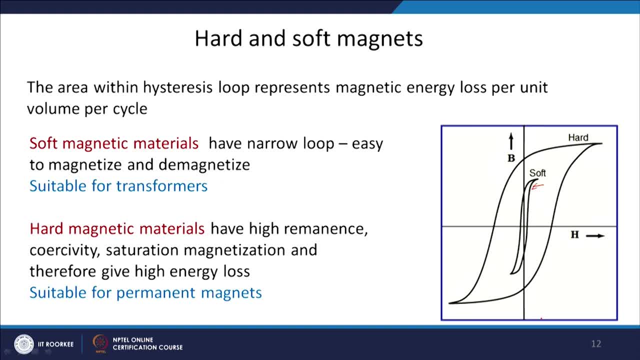 these are actually- that is why- important for transformers. okay, so you can understand: in transformer, okay, you have primary winding. so, for example, suppose you have a transformer like this, so you have primary winding here, okay, and you have secondary winding here. okay, and in the primary winding an alternating current is flowing which has a short term. 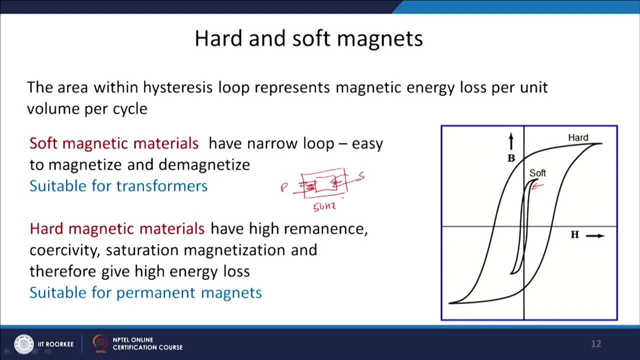 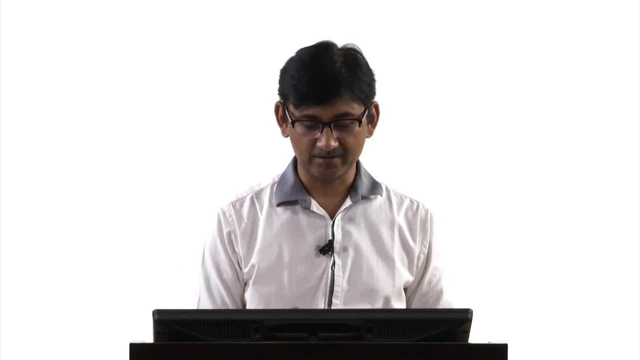 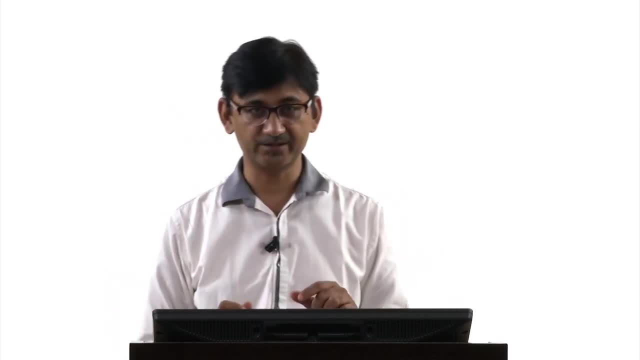 which has a cycle of 50 hertz. okay, that means 50 times it is becoming positive and negative. okay, so my this core material will also get demagnetize. this whole cycle will be repeated 50 times in a second. okay, 50 hertz means 50 times. this hysteresis loop is being: you are 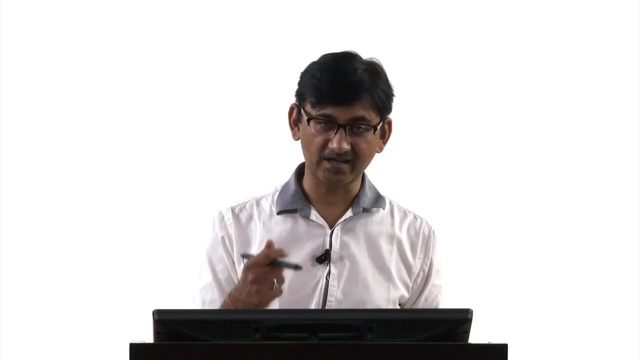 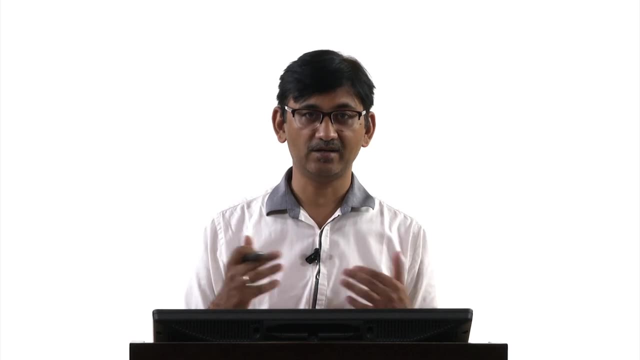 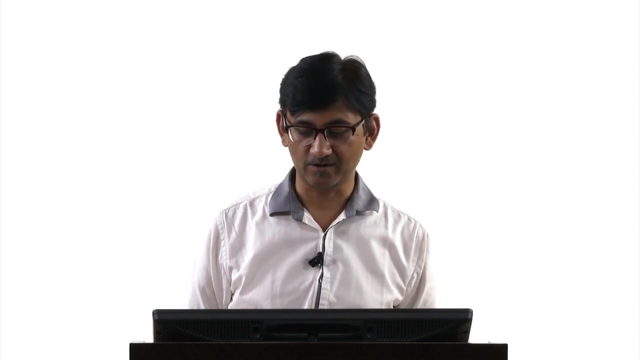 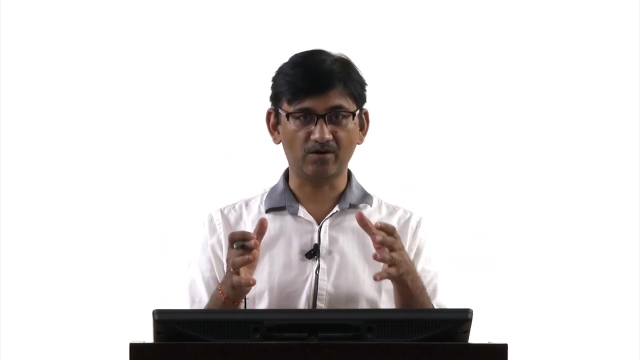 doing in the material. okay, so in each cycle you are losing certain energy. okay, That means there is a big loss of energy during the when the you are stepping down or stepping up the voltage. okay, using transformer. that is why the transformers are covered with oil. okay, they are submerged in oil to take out all this heat. and you must have seen on. 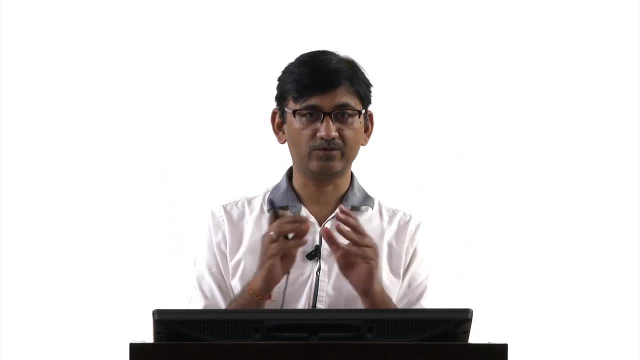 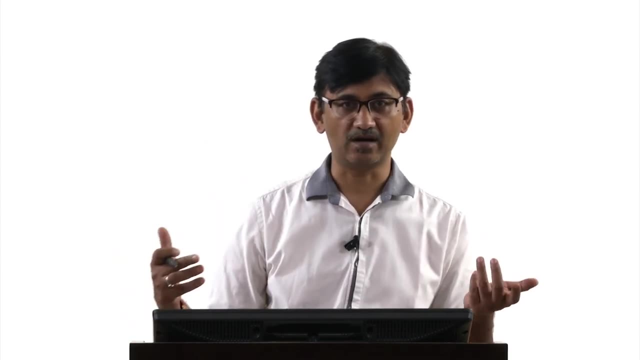 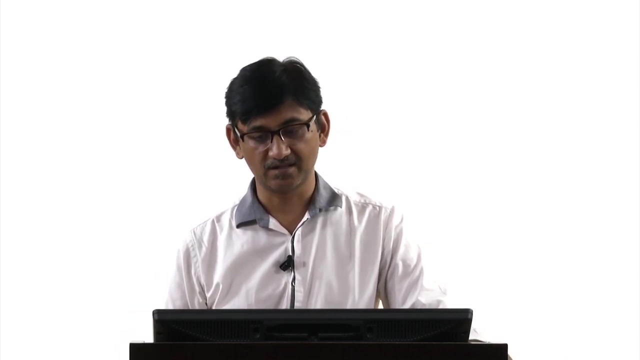 the transformer: outer surface. also there are fins, okay, to increase the surface area so that this heat can be dissipated. Transformation of transformer, And sometime you must have seen that the transformer also burn up. okay, because there is so much heat is generated. so you can understand the importance of hysteresis loop that I have. 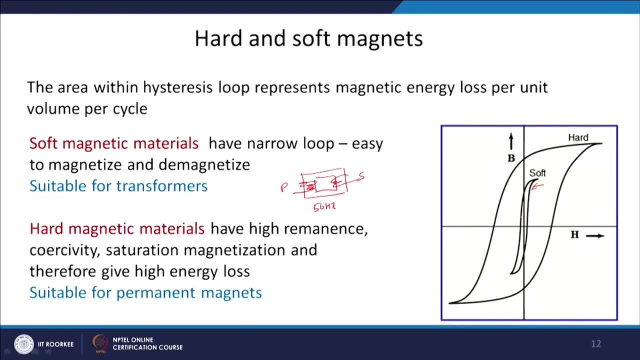 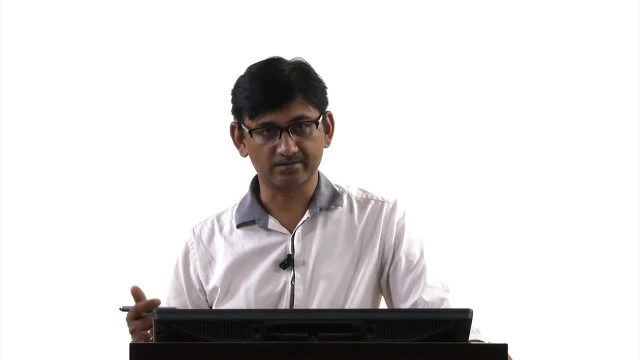 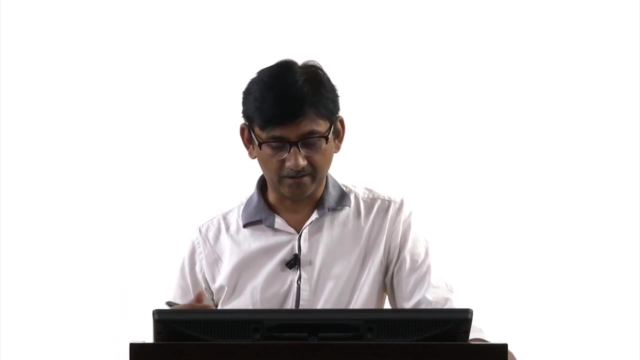 to have material which has a smaller hysteresis loop. okay, and these are called soft magnetic materials. a lot of research goes in the making of this type of material. One of the most important material which is used for this transformer applications are silicon steels, which contains around, I think, 2 to 3% silicon. okay, and they show this kind. 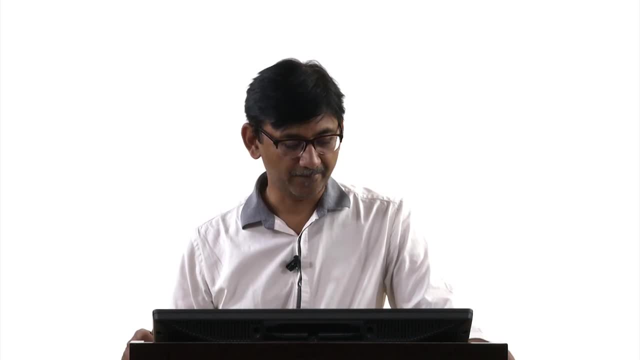 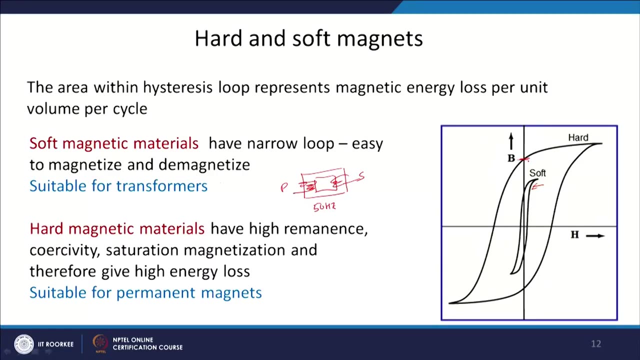 of soft magnetic properties. okay. Now hard magnetic materials are also important. okay, they of course have high remnants. okay, they have higher coercivity saturation. magnetization will also be higher. okay, and that is why they have higher loss of energy. but for materials where you do not want to keep changing their, 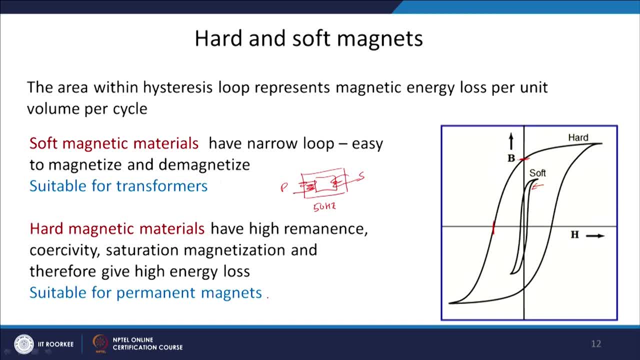 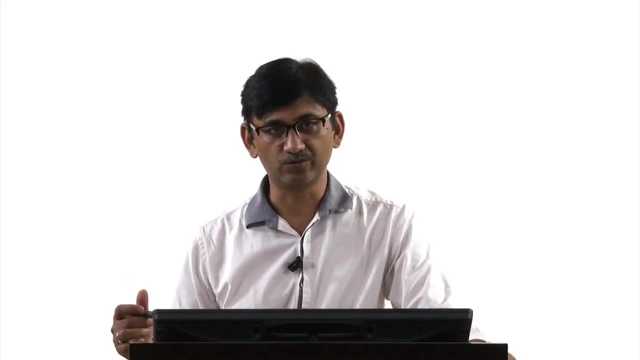 magnetization condition: okay, these are important. so in permanent magnets we will use hard magnetic materials, because in these material, once we have magnetized it, we want it to remain like that, okay, So if it has a higher saturation magnetization, then it is good. the magnetic field which it 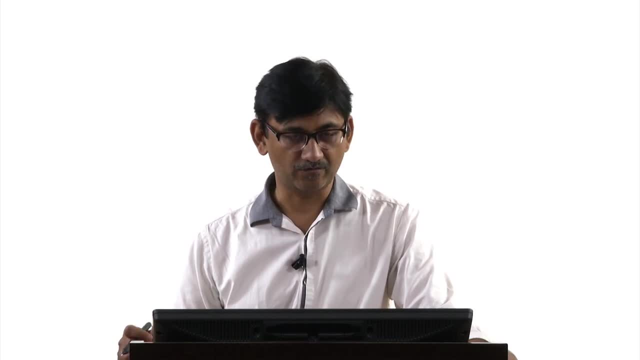 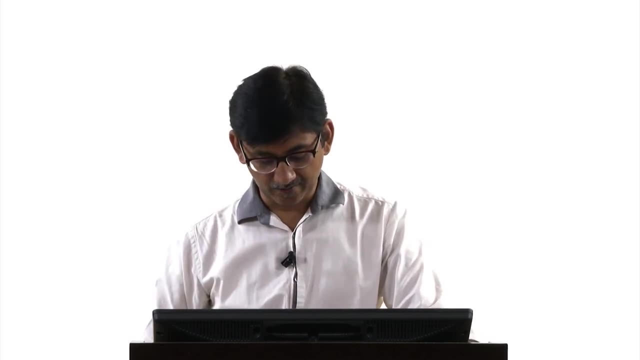 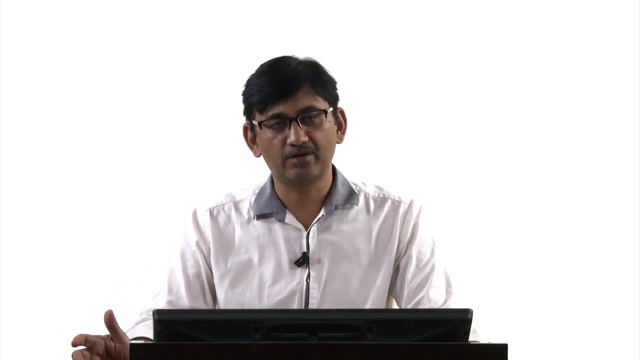 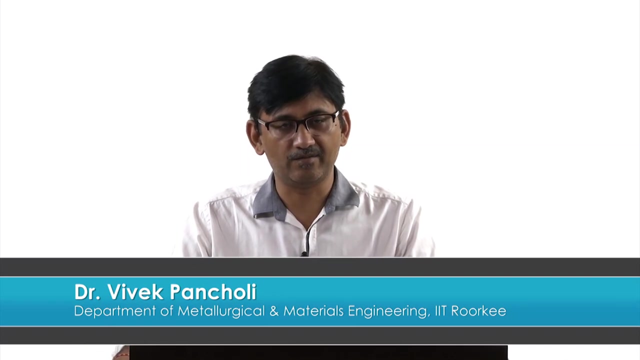 is going to generate, So it will be of higher value. okay, so for permanent magnets, we want to have hard magnetic materials. So with that we have covered two very important class of materials: electrical magnetic materials. okay, and we have seen few properties of these materials, which are of great importance to